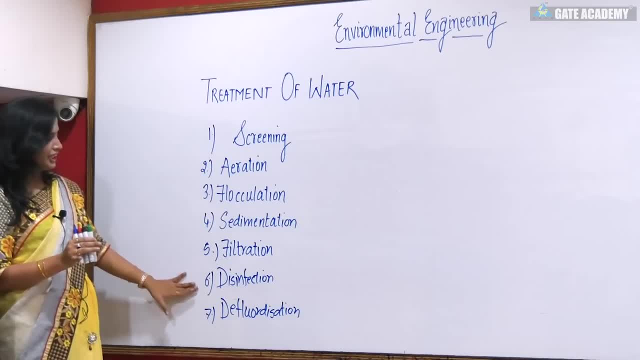 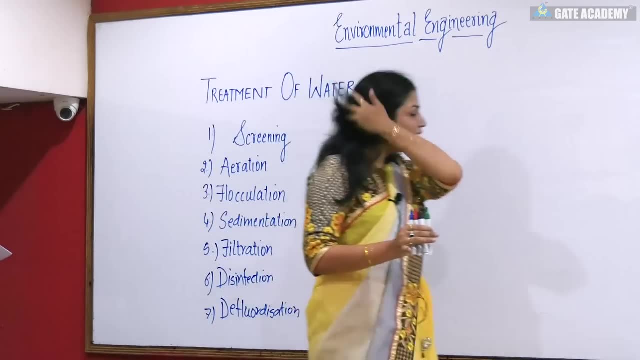 aeration, flocculation, sedimentation, filtration, disinfection and defluoridization. We will also deal with the coagulation part also Now, instead of explaining it here, I will be dealing it separately, each treatment unit. Now, first comes the de-fluoridization, So we will be dealing with 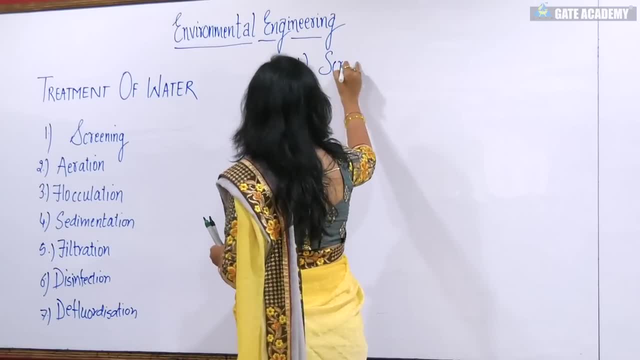 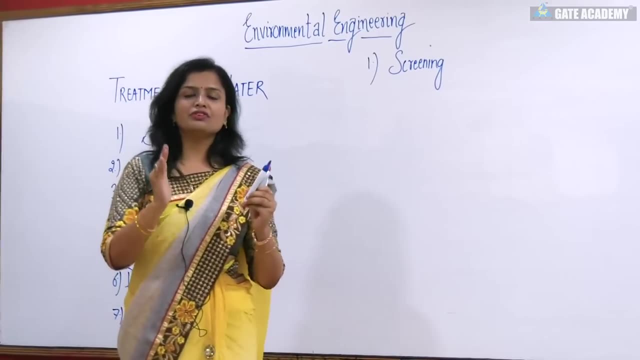 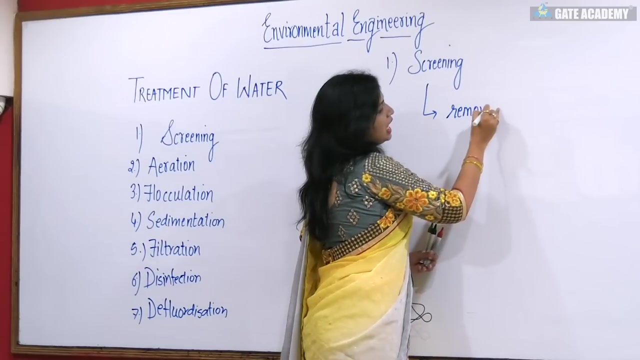 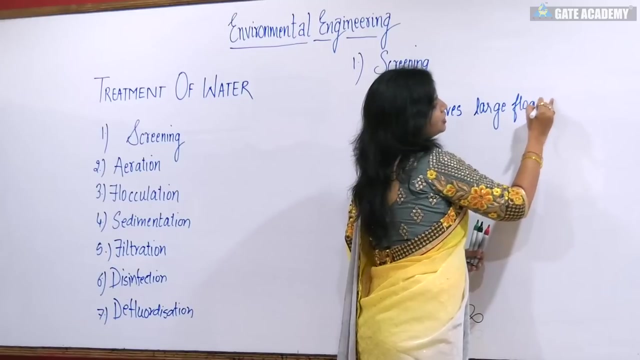 the de-fluoridization. So first comes the screening part. What is screening? And this is the first part of the treatment unit. Why? Because it removes large suspended particles, or we can say: large floating matter Removes large floating. 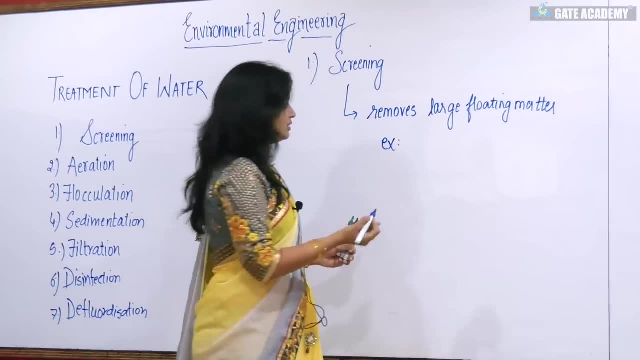 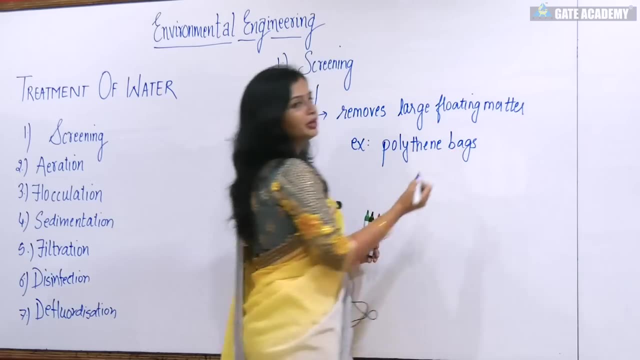 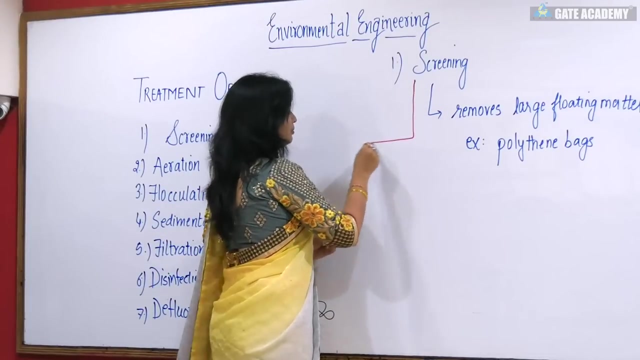 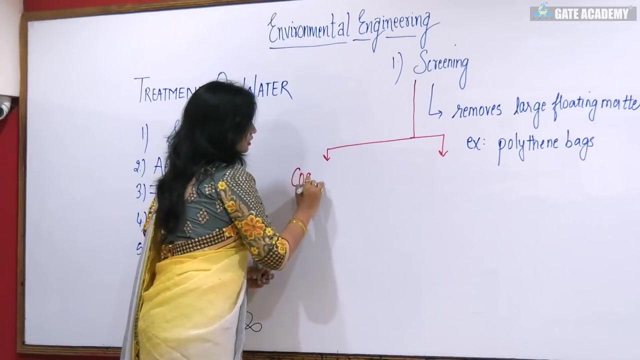 particles. Example could be your like paper bags, your polythenes, etc. which are floating in the water. This can be removed by screening. Now, screening are basically of 2 types. We will divide this screening into 2 types. 1 is the coarse screen and 2 types of the fine. 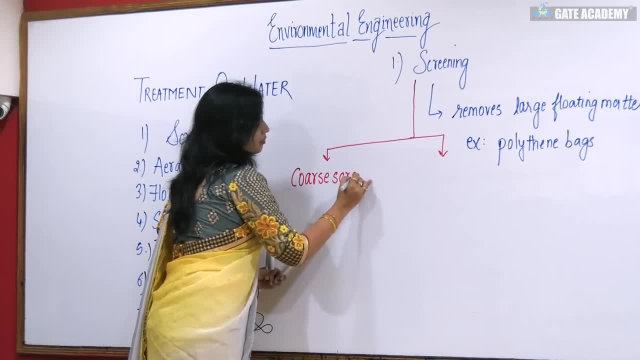 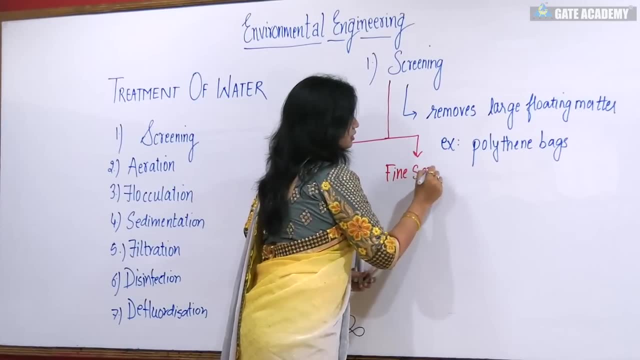 ground. What is coarse screening? The coarse ground is the surface of the skin. This is the surface of the body, The surface of the body, this is the surface of the skin. So the coarse ground And the other one is the fine screen. 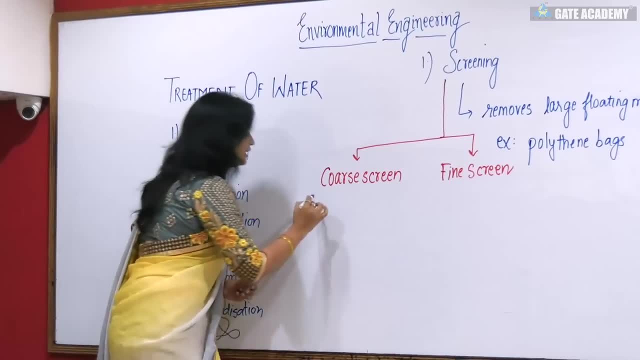 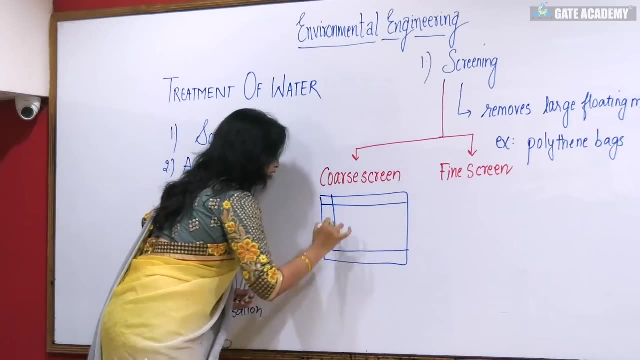 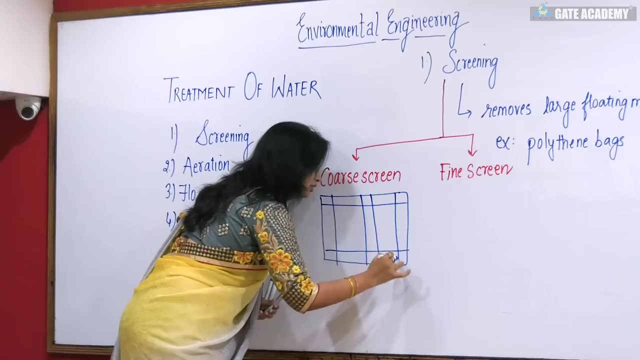 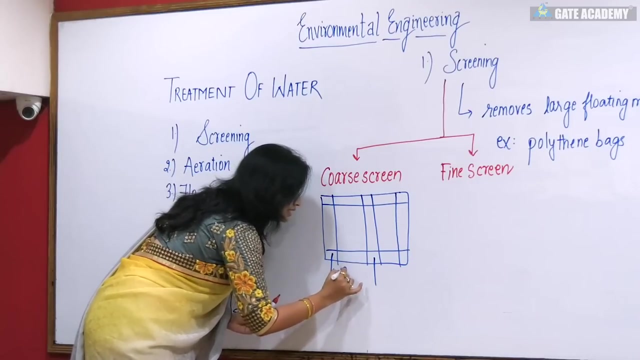 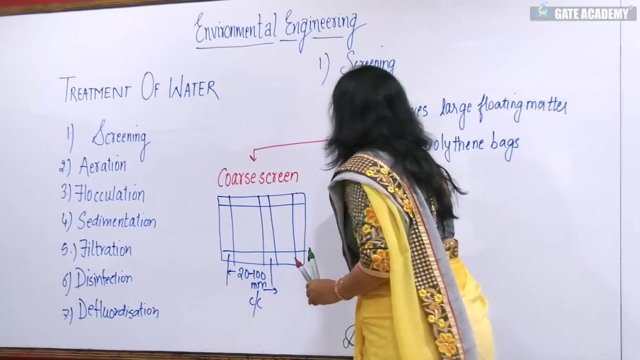 Now the difference between the two is the coarse screens looks like this: They are spaced at equal intervals. Now the distance between the bars is 20 to 100 mm center to center. when we use the coarse screen, Fine. Similarly, when we use the fine screens, fine screens have very minute pores in them, as 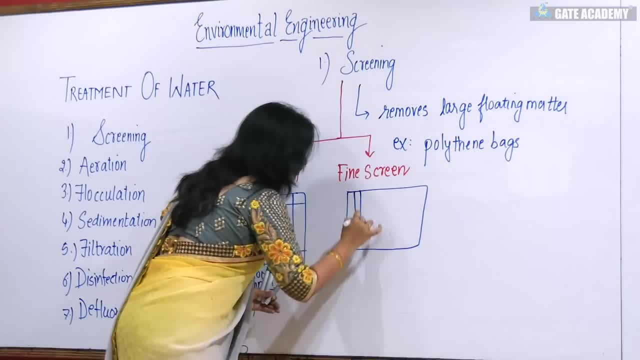 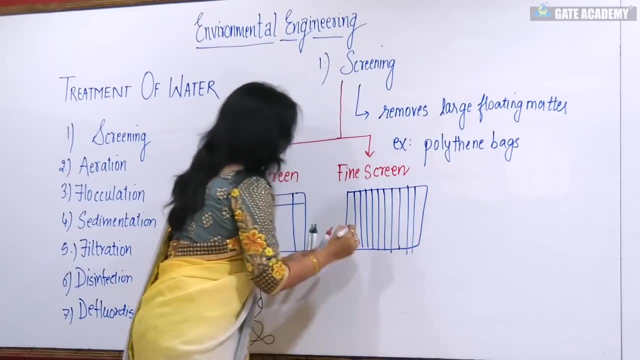 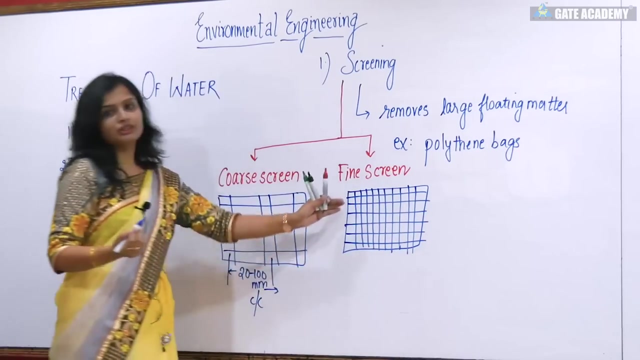 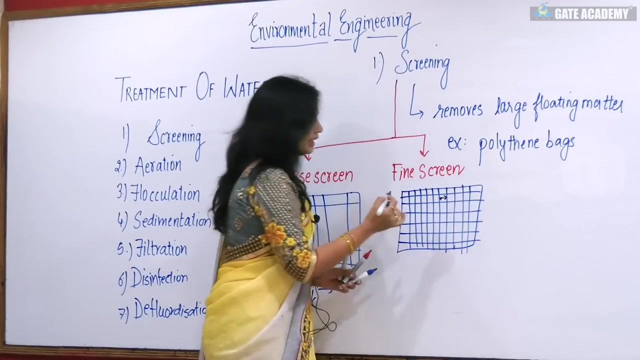 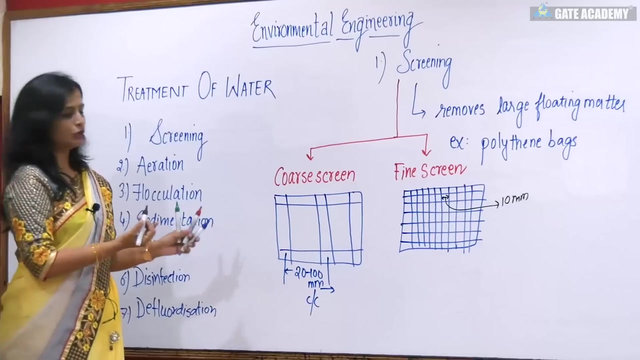 the name suggested, I will draw this fine screen having very minute pores. Okay, So this is the fine screen and this pores. the size of this pores, or we can say the mesh, is 10 mm. 10 mm is the size of the pore or the mesh opening, while here we have provided 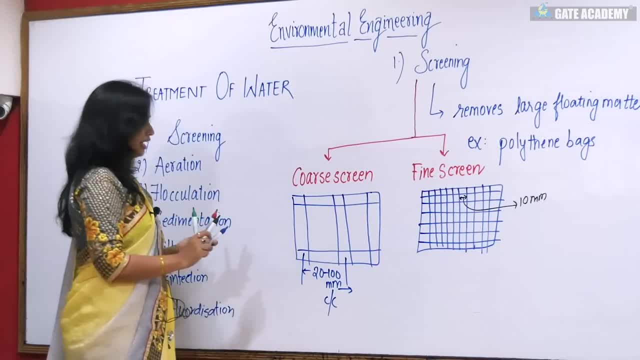 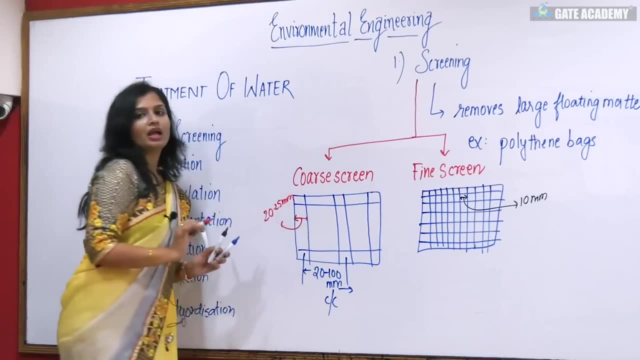 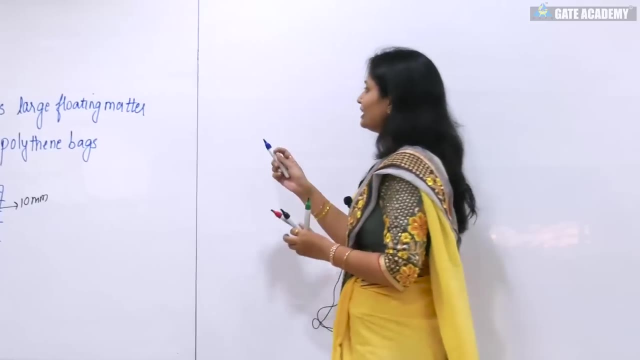 the coarse screen. So the distance between center to center is 10 mm. Okay, So the distance between center to center is 20 to 100 mm, and the dia of the bars is generally 20 to 25 mm. Now how is the screen placed in while the treatment of water is done? 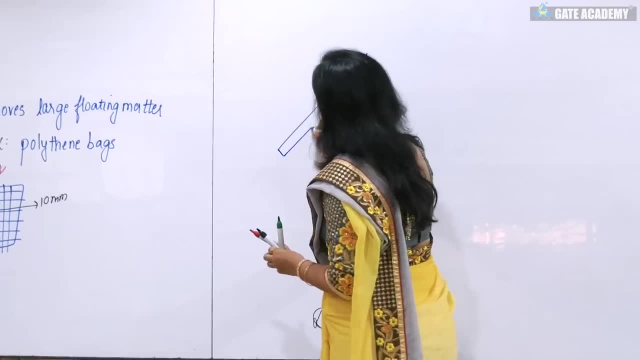 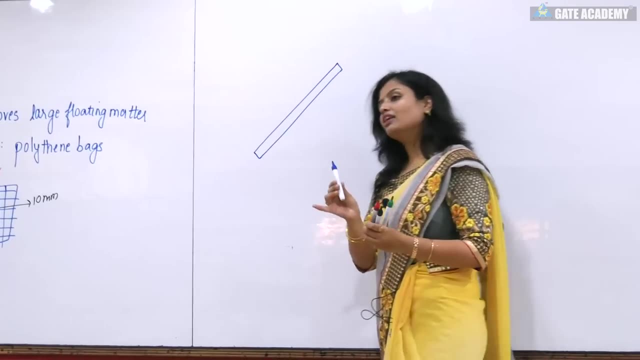 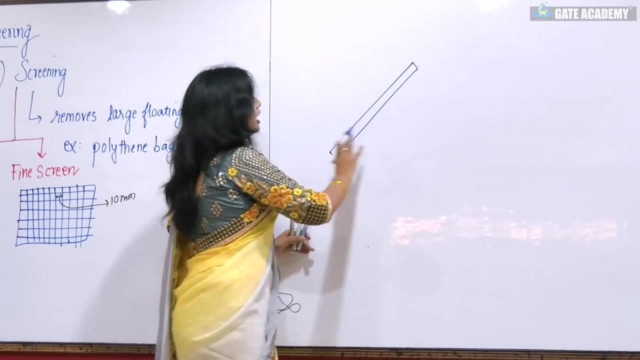 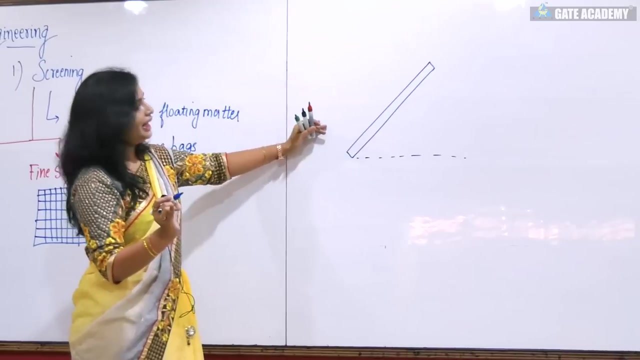 Screens are generally placed inclined to the flow of water. This is the screen and it is placed in a inclined way. What will happen, and what is the logic of placing it in an inclined manner, is that, while you place them in this manner, you will see here, like you can see here, the velocity. 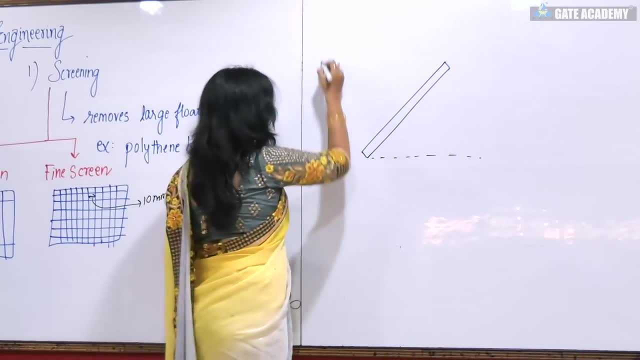 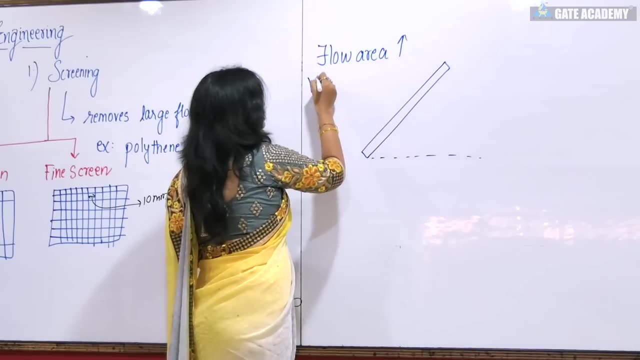 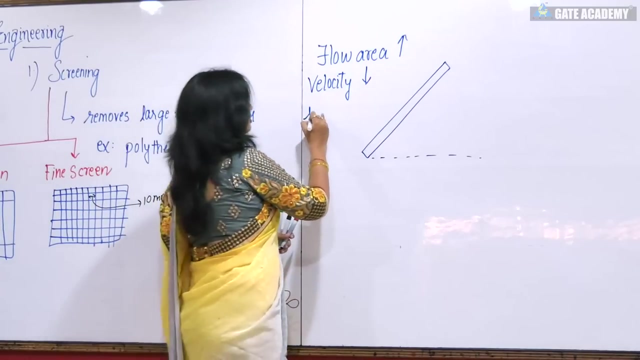 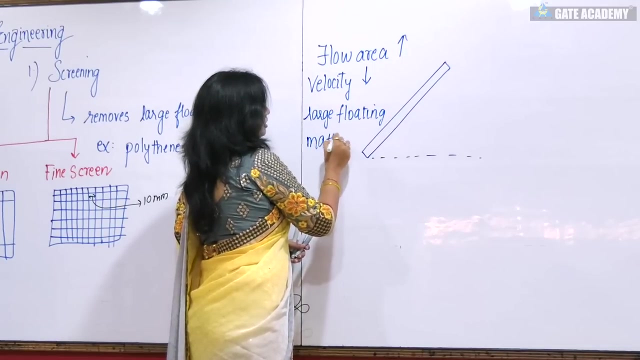 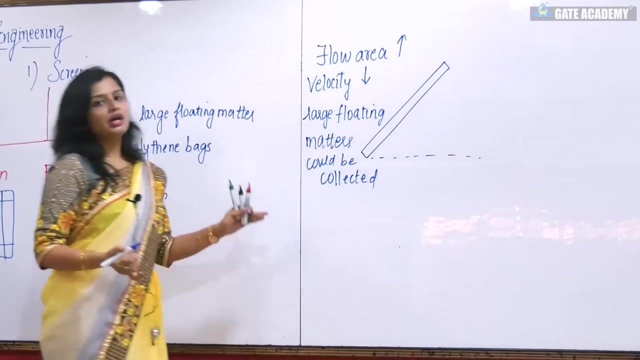 the area will increase. the flow area will increase. flow area increases, velocity reduces and, because of this, large floating matters could be collected. Okay, Okay, Okay. Now the question comes: who is more efficient? coarse screen is more efficient to be used. 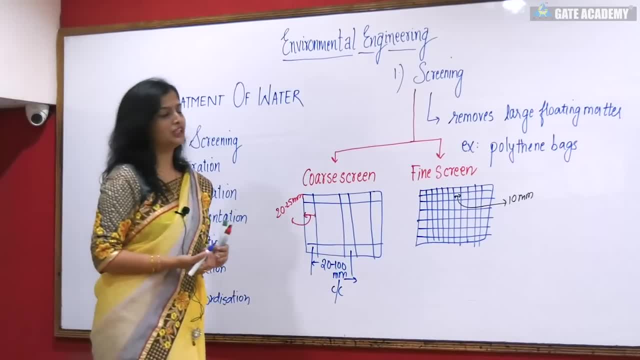 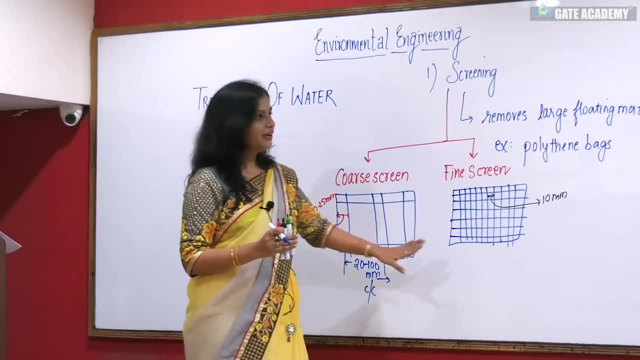 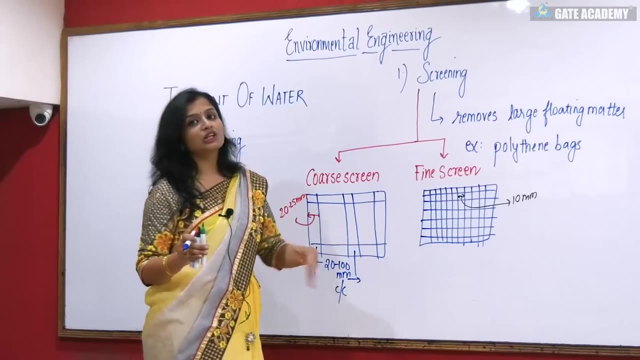 or fine screen is more efficient to be used. Actually, for treatment point of view, we prefer coarse screen as compared to the fine screen. Reason: Fine screen has small size of the mesh opening- Okay size of the mesh opening- because of which it gets clogged very frequently and because 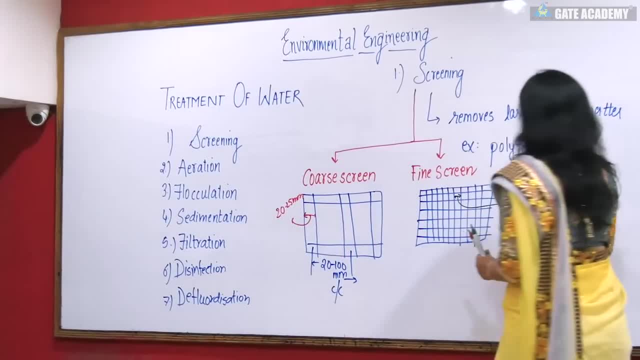 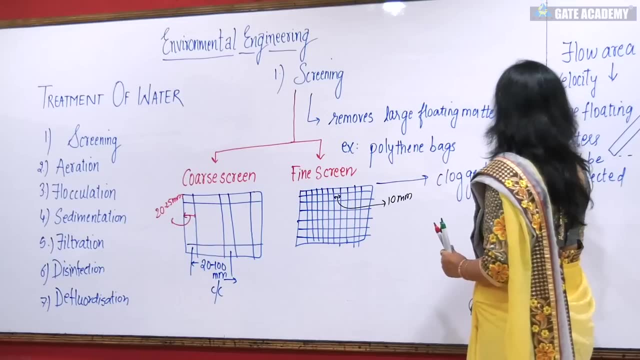 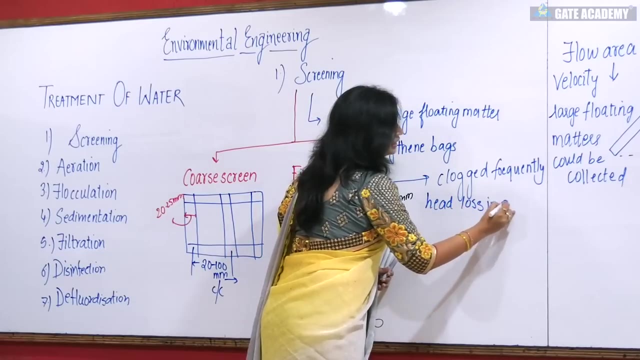 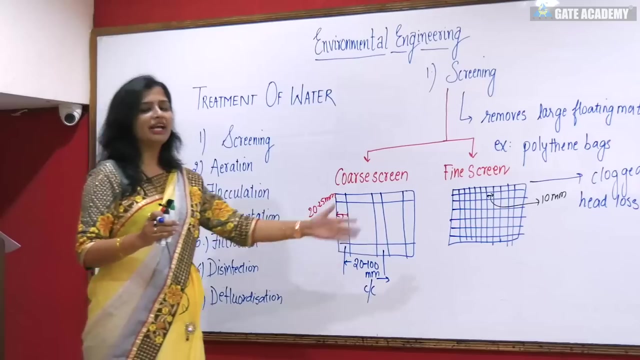 of it. also, the head loss increases. What is the point? It gets clogged frequently due to its smaller size of the pores and head loss increases. That is why we try not to remove the minute particles from the fine screen, the fine suspended particles, so that we can remove them in the sedimentation tank. 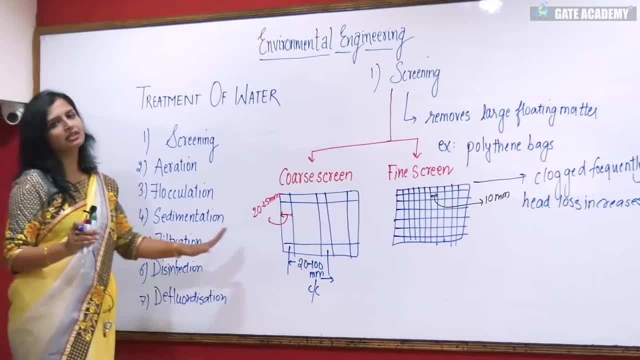 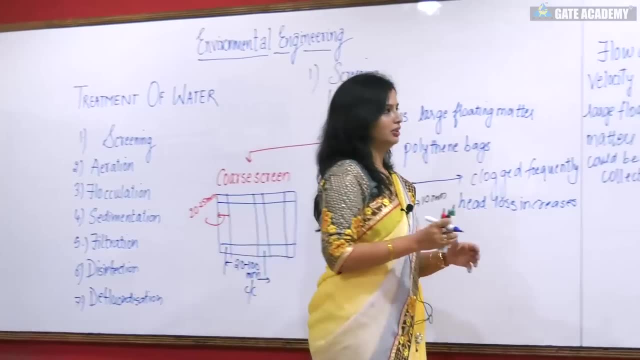 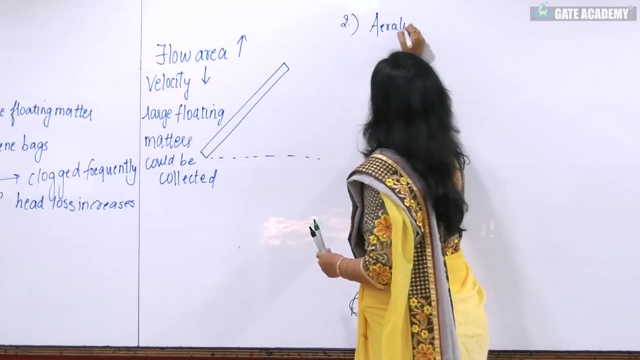 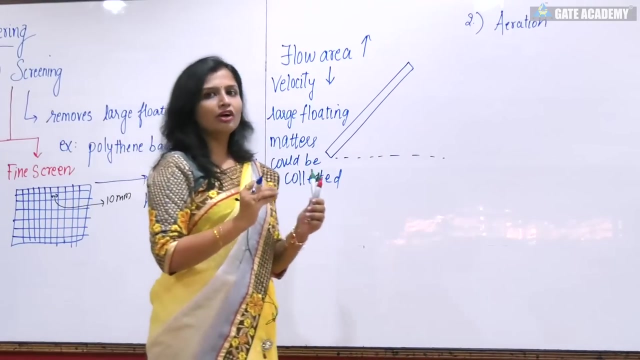 The basic aim is that the large suspended particles or floating matter gets removed in the coarse screen. Fine, I hope you are clear with this. Now we will move to the aeration part. Now, this aeration word, which you would have related to supply of air, that is, supply of 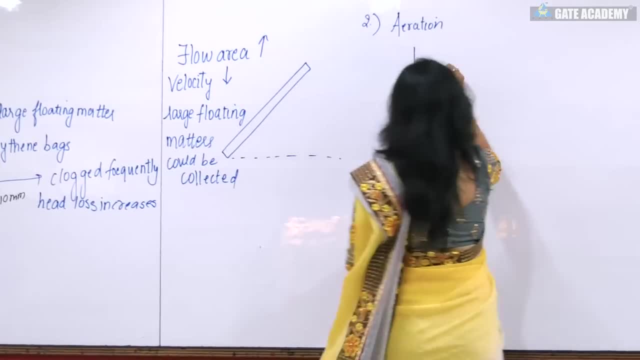 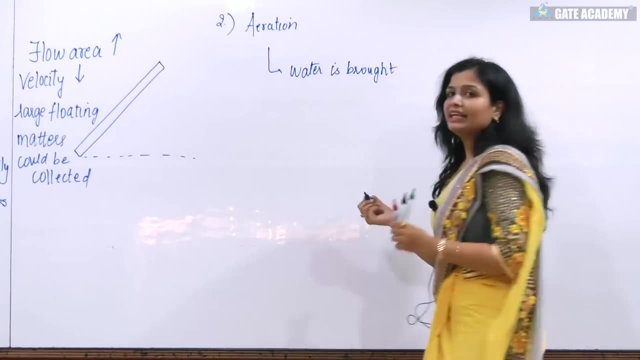 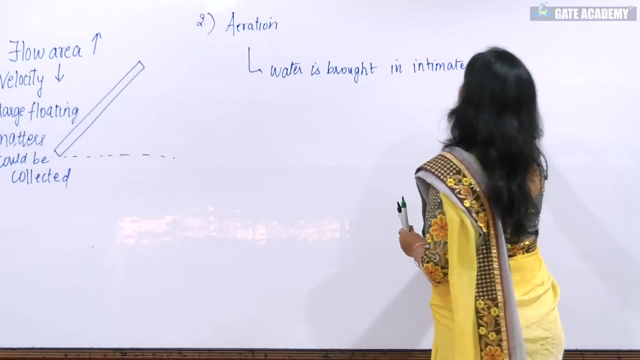 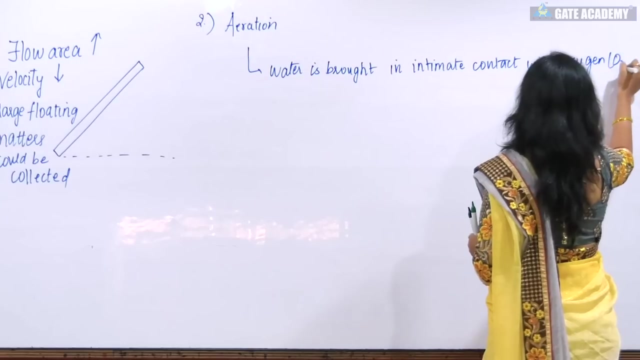 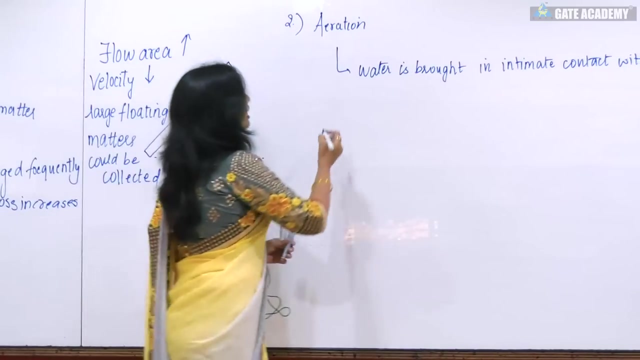 O2.. So aeration is when water is brought. water is brought in intimate contact with oxygen. Intimate contact with oxygen, That is the O2.. That is known as aeration. Now what is the need to do? aeration, because with the help of aeration we can remove odour. or we can remove odour, or we can say gases like carbon dioxide and hydrogen sulphide. Similarly, With the help of aeration, Fe2 plus ions could be removed. However, when we give oxygen to Fe2 plus ions, they generate H plus. When we give oxygen to it, we supply oxygen, although it precipitates, but then also it. gives H plus ions, because of which the concentration of H plus ions increases and naturally the acidity of water will increase. So this is the aeration part, but in aeration we do not have to study only this. We got to know that it removes odour gases. it removes metallic compounds like Fe2 plus. 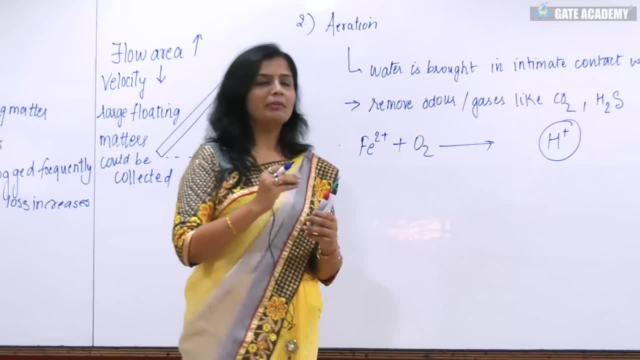 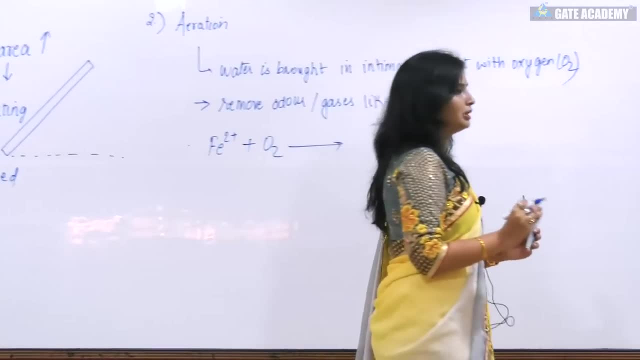 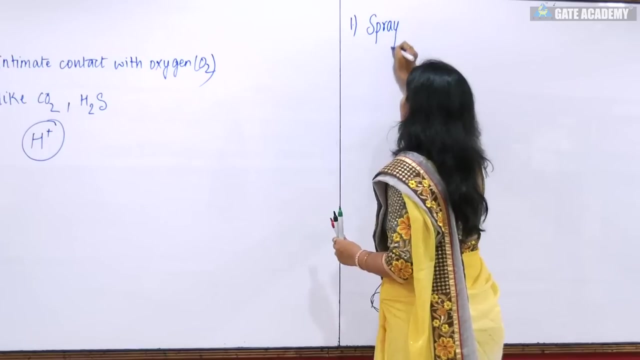 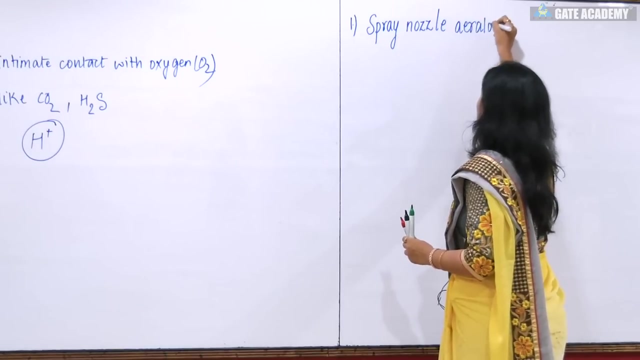 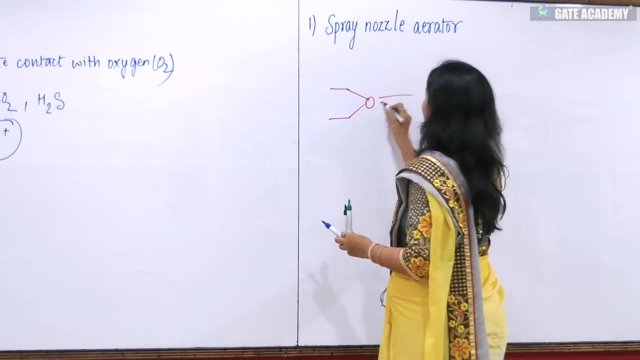 it precipitates it. But there are various other measures, or we can say there are various ways by which we can provide aeration. There are various aerators, to be specific. Now, the first aerator is spray nozzle aerator. Here, what we do it, this is some sort of spray and we are ejecting water. or we can say we 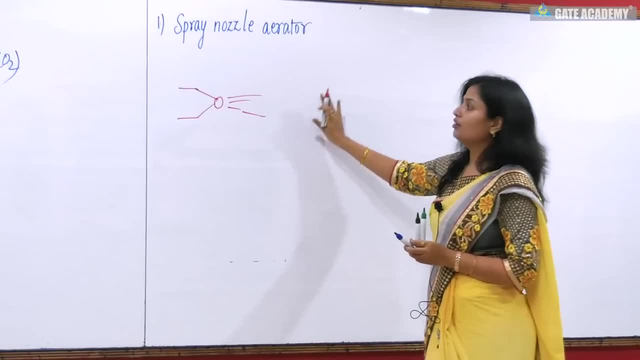 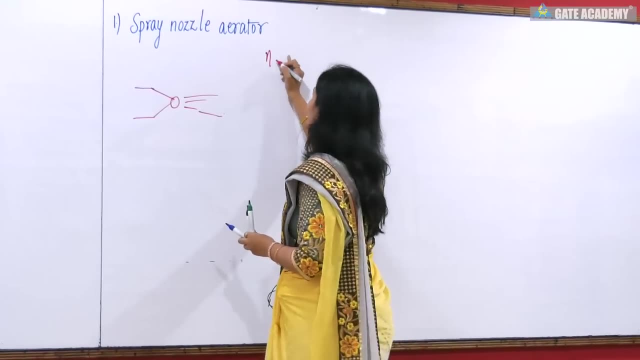 are providing. with the help of the pumps and supplies we are providing, we are making the water to come in contact with the oxygen. However, this is very efficient. It is efficiency for removing carbon dioxide, So this is very efficient. So this is very efficient. 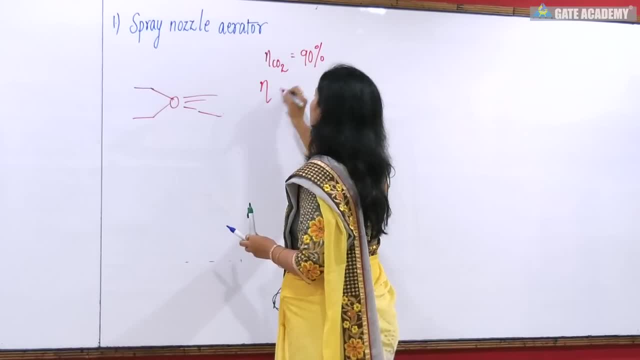 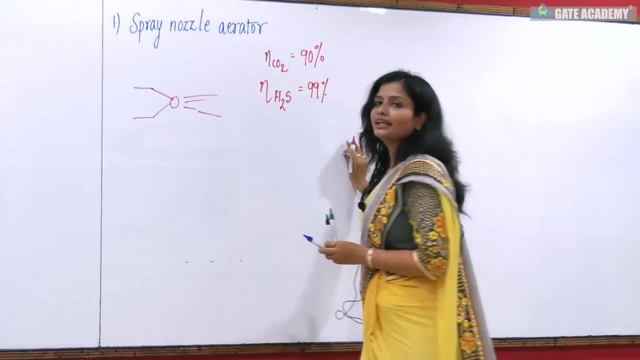 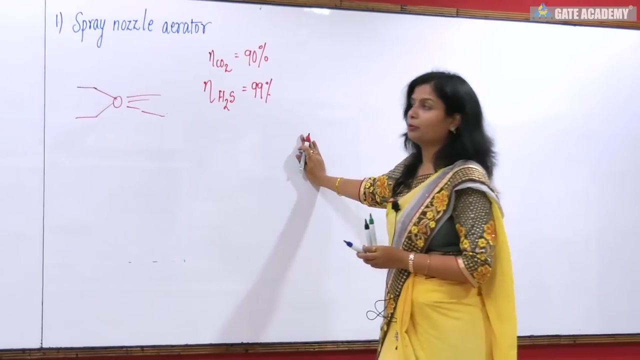 Again, it is 90%, and for H2S gas it is 99%. So this is a highly reliable source, but it is very costly and so, basically, we do not use such sort of source because of economic point of view. Now I have drawn a diagram of the spray nozzle for you to understand. 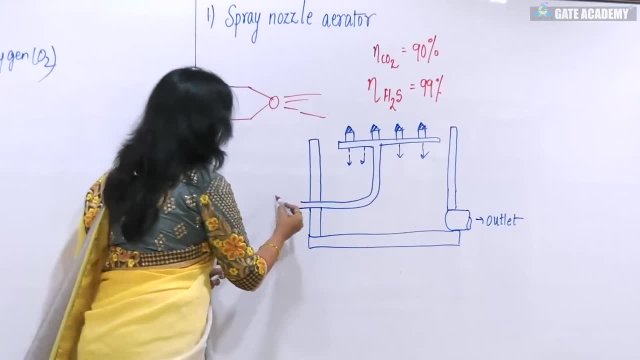 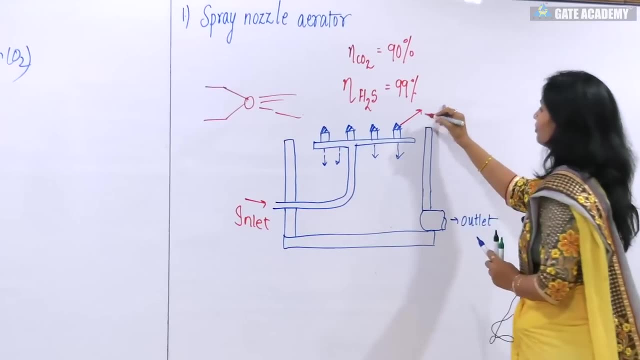 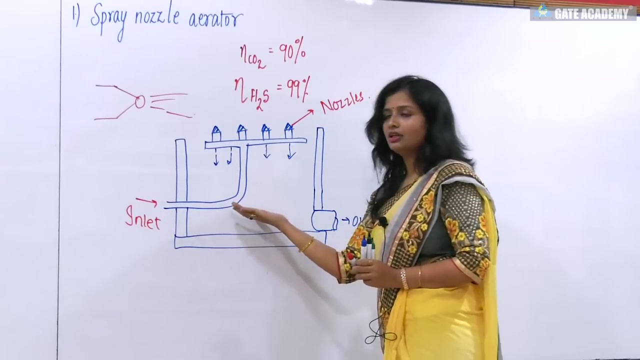 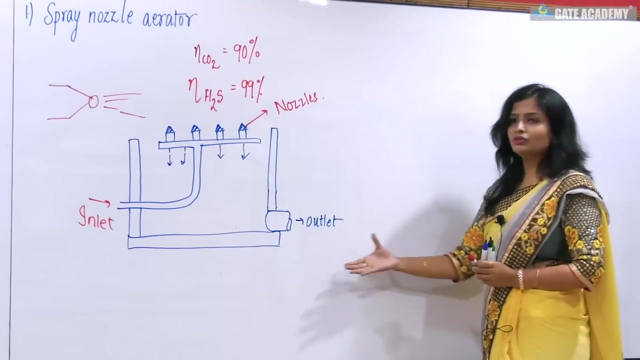 Like this is the inlet part of the water And these are the nozzles. nozzles which is provided, fine, So the water is made to enter through here, then from the nozzles they just come in contact with the oxygen and after which they go out through the outlet pipe. 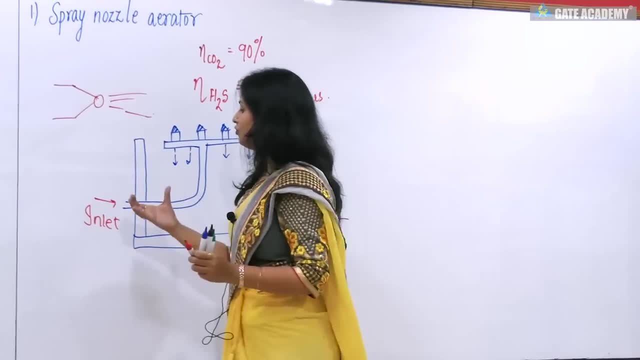 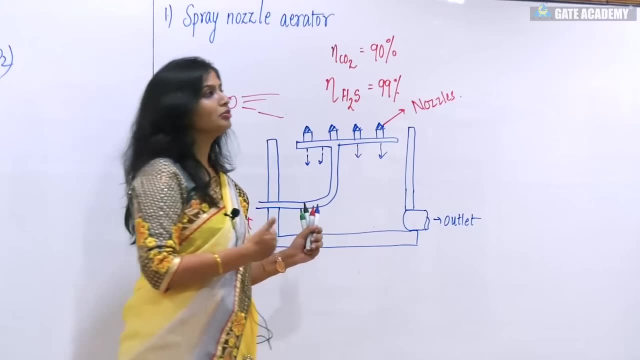 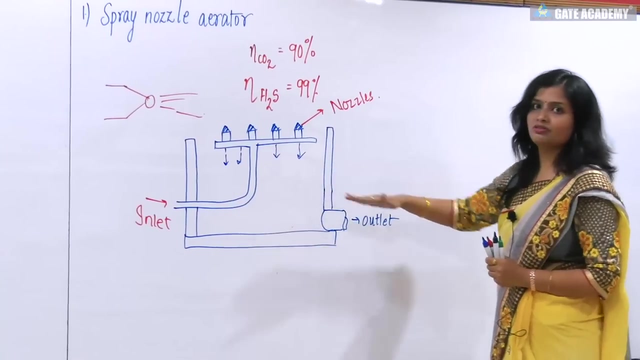 Here what is happening: for water to eject down or water to be supplied at a height, You will be needing what? You will be needing: some sort of energy, or we can say some sort of mechanical, mechanically supplied energy so that it could travel this part- motors, we can say. to be specific, 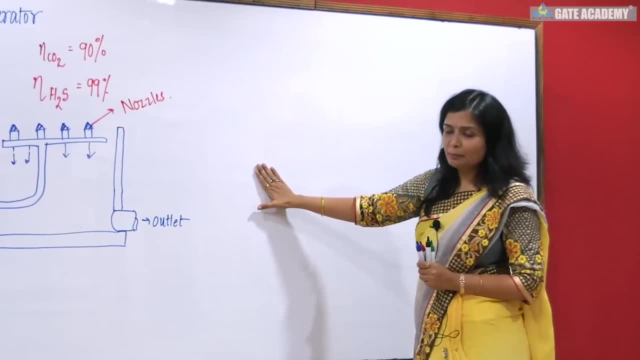 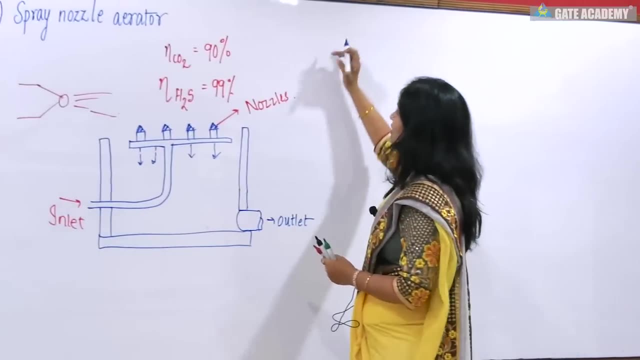 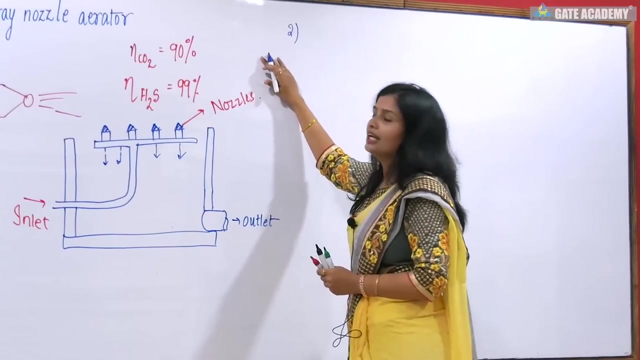 So this is a costly process and, basically, as per economic point of view, although the efficiency is good, but we do not use it. After this comes the cascade aerator. however, you have to learn the efficiency that for carbon dioxide it removes up to a 90 percent. 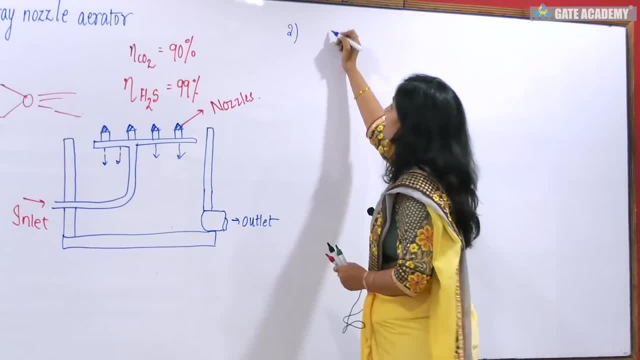 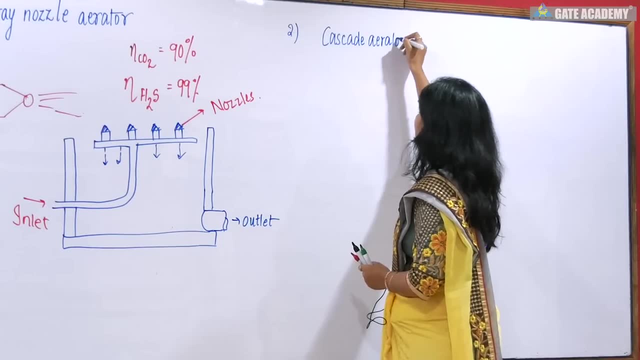 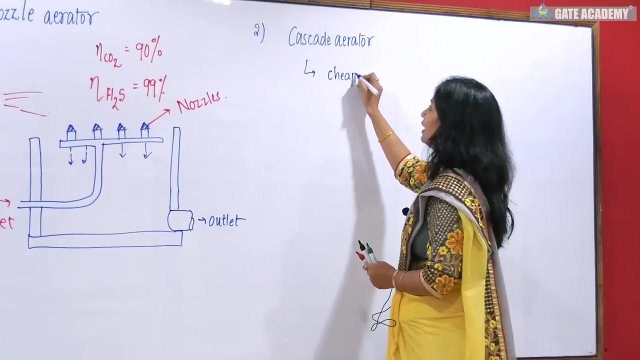 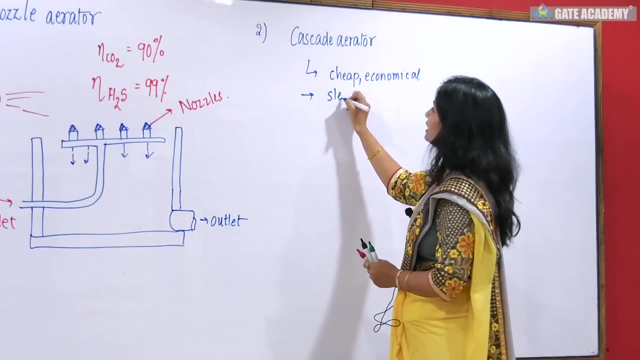 And hydrogen sulphide. it removes up to 99 percent. After this comes the cascade aerator. The advantage of this aerator is it is cheap, economical and this tips which is being made, tips of cascade aerator, are made from carbon dioxide. 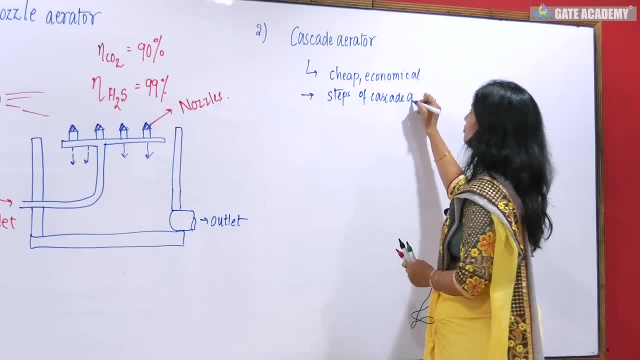 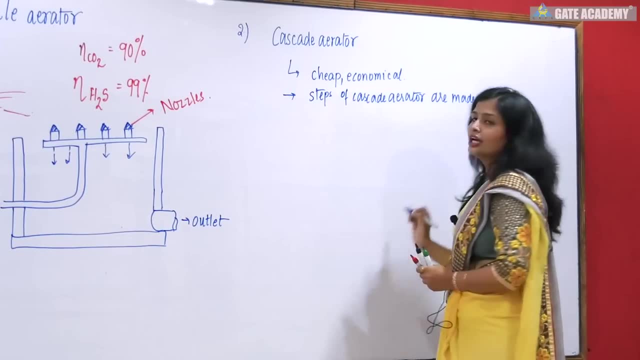 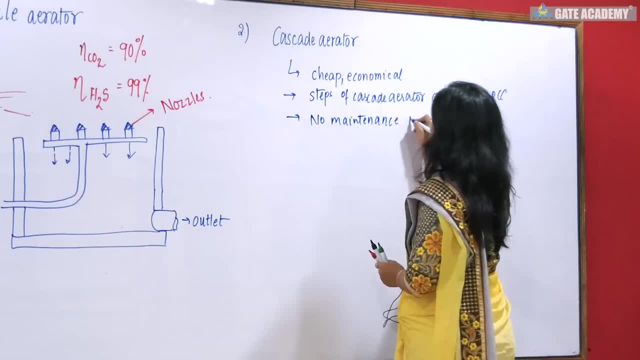 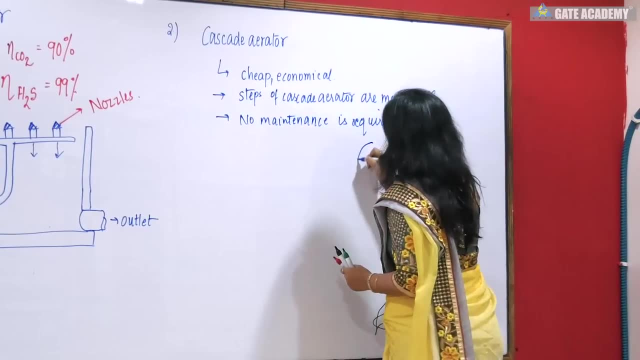 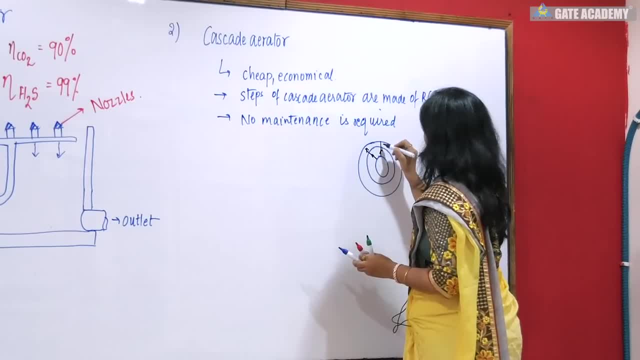 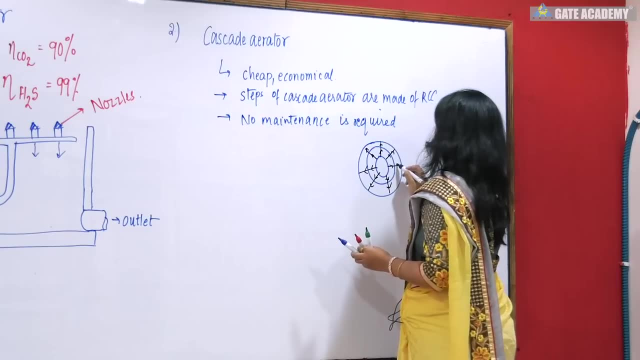 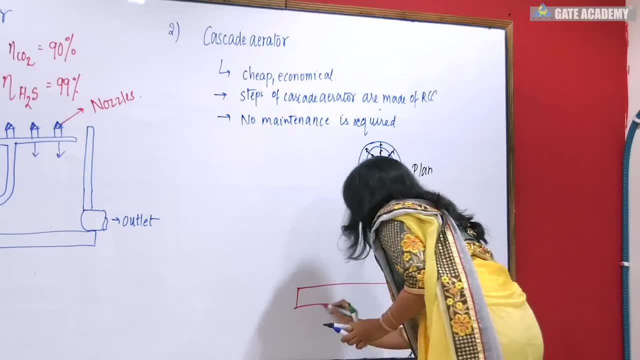 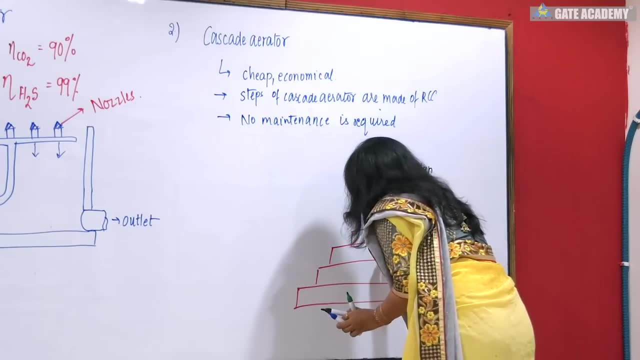 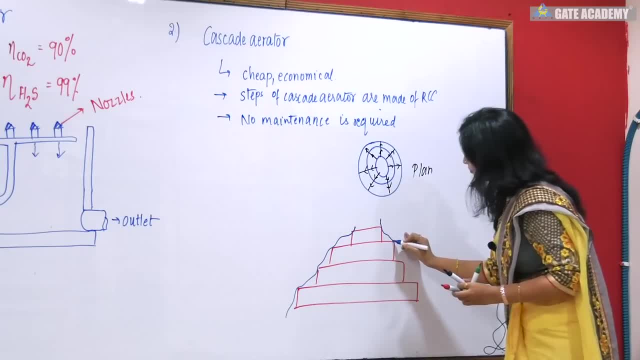 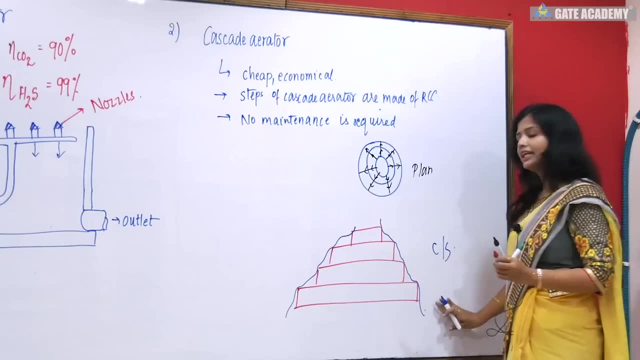 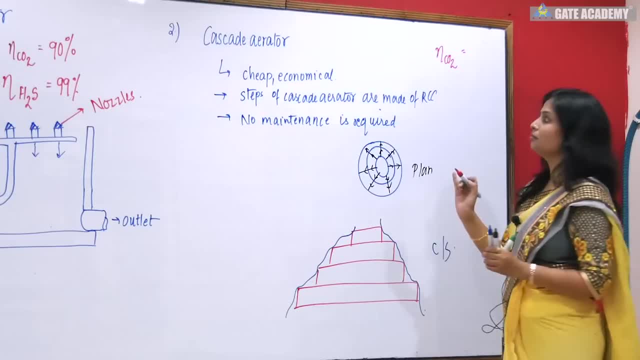 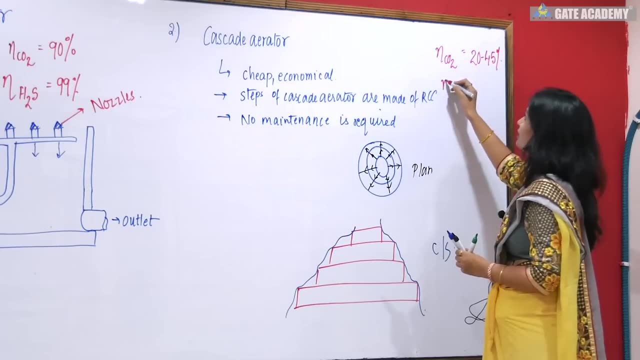 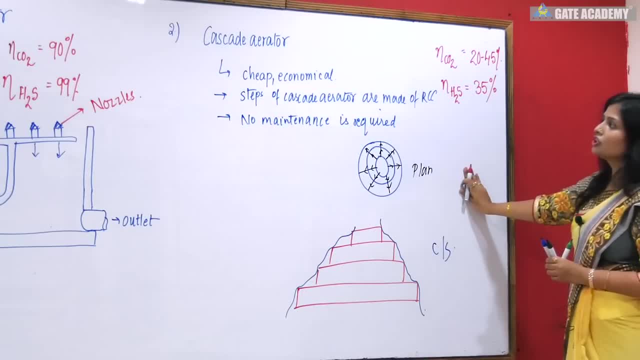 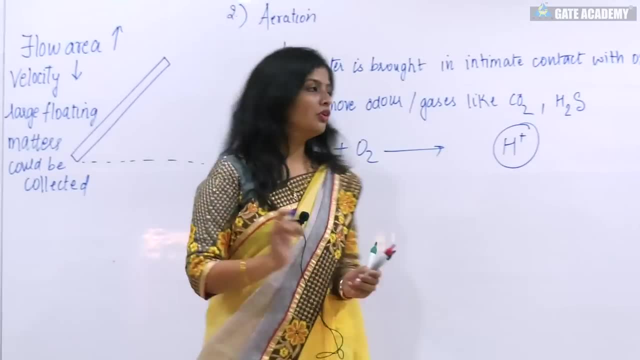 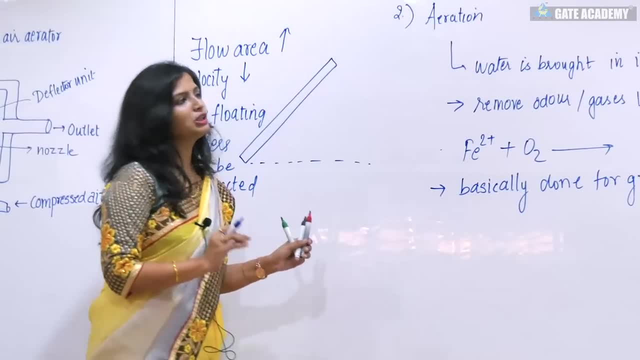 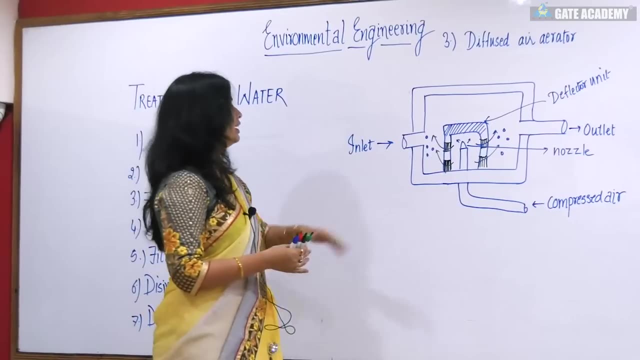 It was the second which we discussed. now, coming back to the initial one: spray nozzle aerator, cascade aerator- Third will be the diffuse air aerator. I have drawn the diagram for you to understand. This is the inlet where the water which has filtered, or we can say when the large floating. 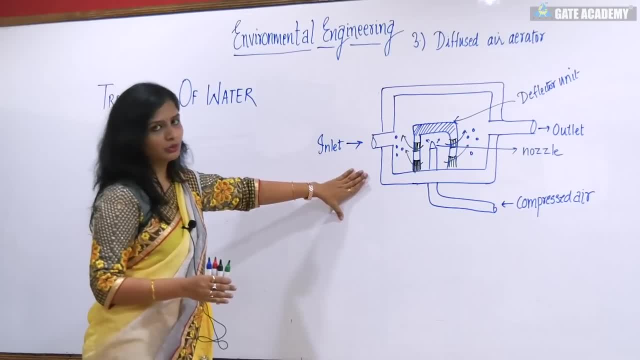 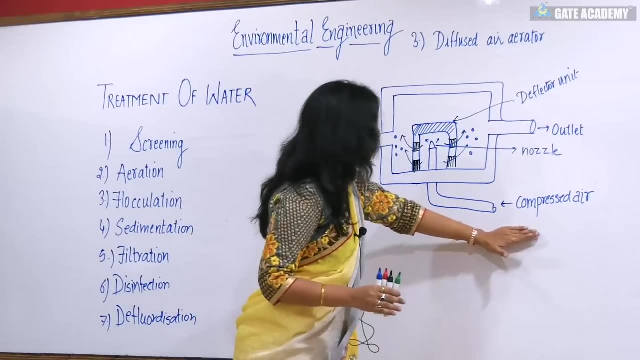 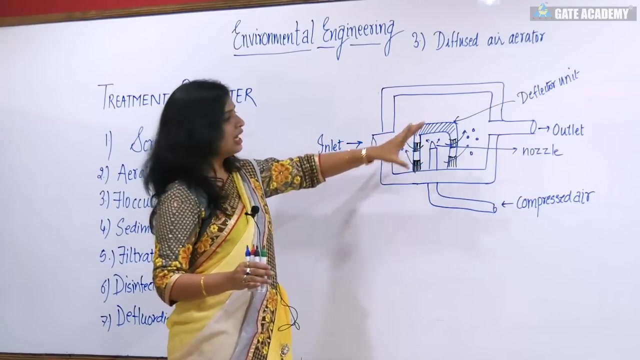 matter have been removed from the screening is made to enter through the inlet This waste water. when it comes, we can see this chamber. the compressed air is made, is allowed to flow through this and with the help of nozzle, it is spread. This is the deflector unit. 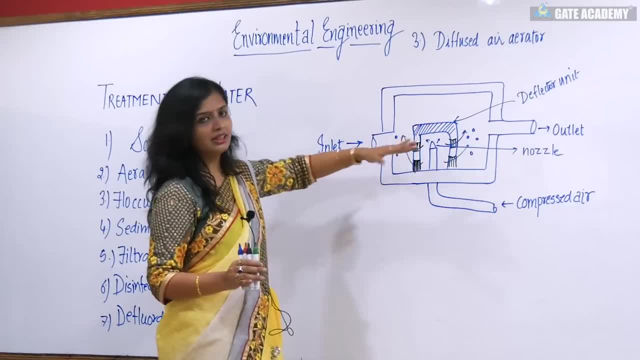 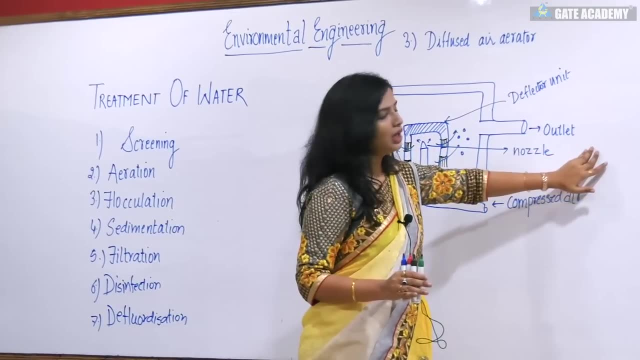 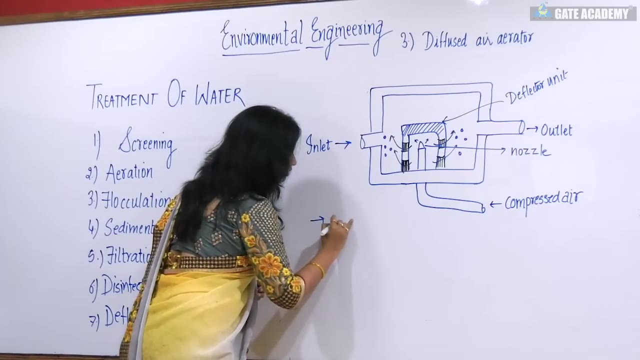 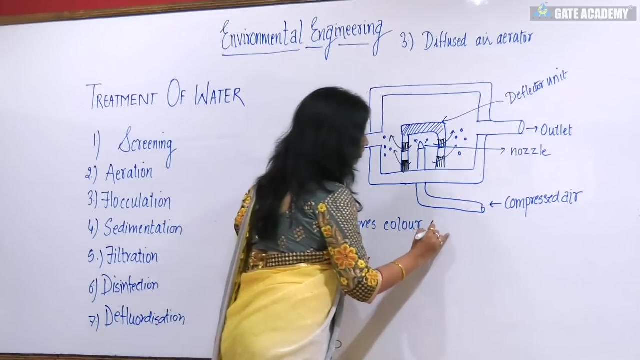 So when this compressed air moves, it starts to deflect the air, And so the water comes in contact with the oxygen, after which it discharges through the outlet. So this was the diffuse air aerator. What is the main use? It removes colour and odour of water. 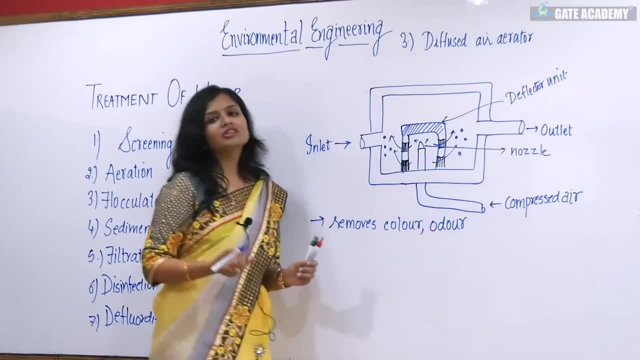 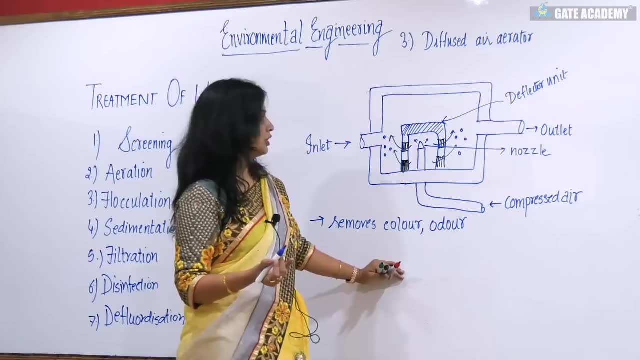 You can see multiple colours in water due to the presence of any algae or due to presence of any harmful substances. So it removes the colour, Okay, And the bad smell which comes in the water. So basically, we use diffuse air aerator. it is also costly. 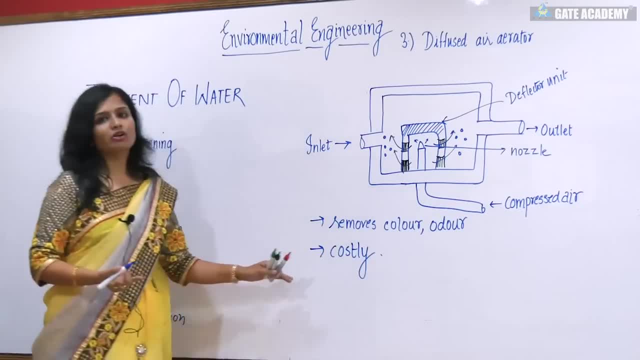 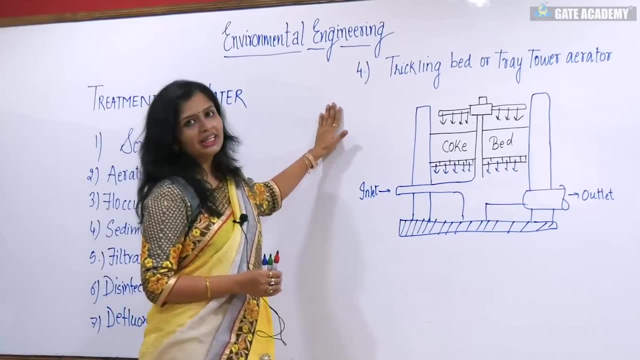 Because supplying of compressed air deflector units, it all is very costly. Now, after this, we will be seeing the trickling bed filter. After this, we will be studying the trickling bed or tray tower aerator. What happens is basically first understand why we use this. 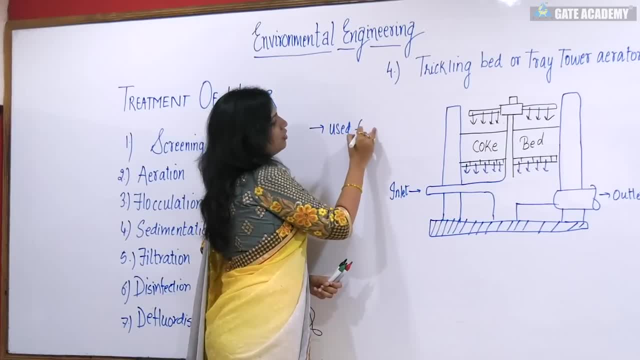 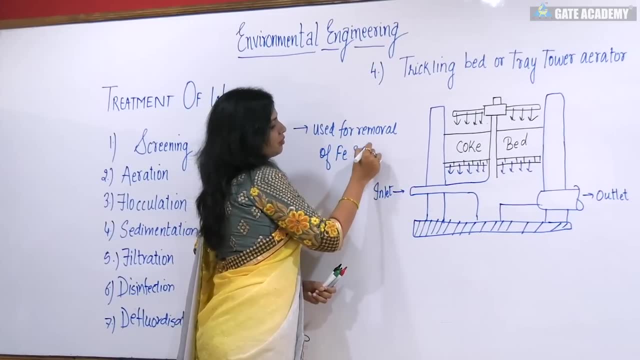 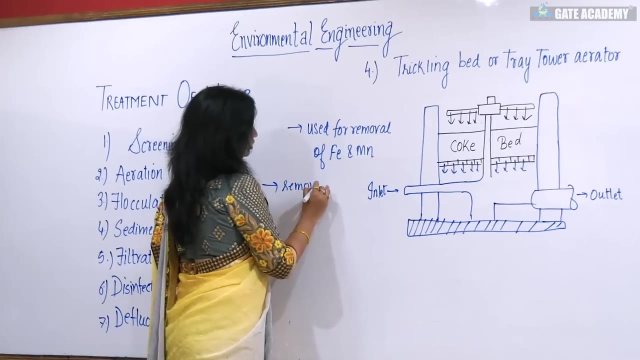 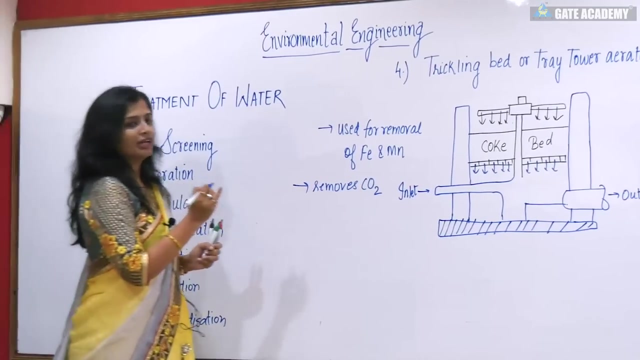 It is used for removal of the air. Okay, This is the deflector unit. This is used for iron and manganese, first of all. This is very much helpful in removing carbon dioxide from the water. removes carbon dioxide Fine. Where we use this trickling bed filter or tray tower aerator. 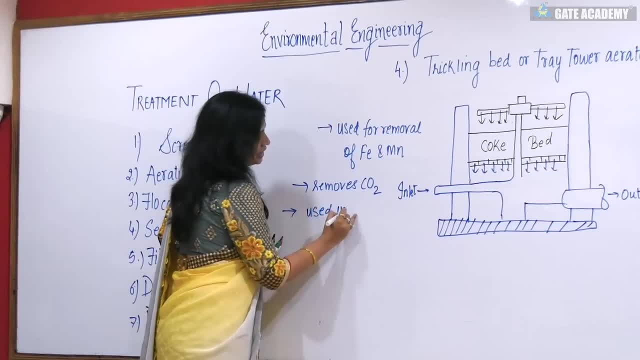 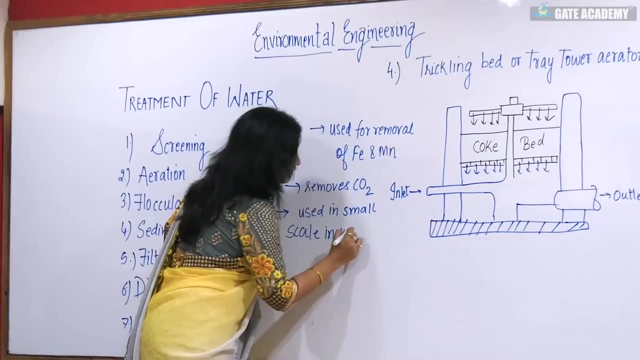 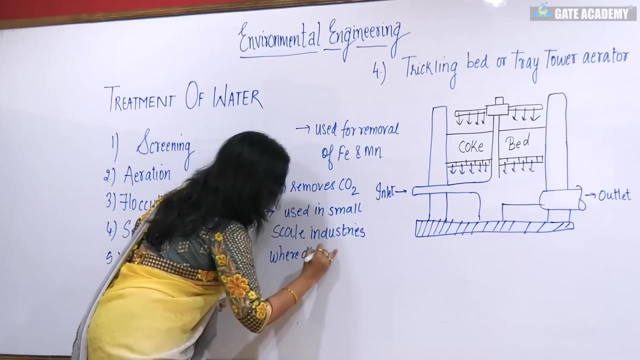 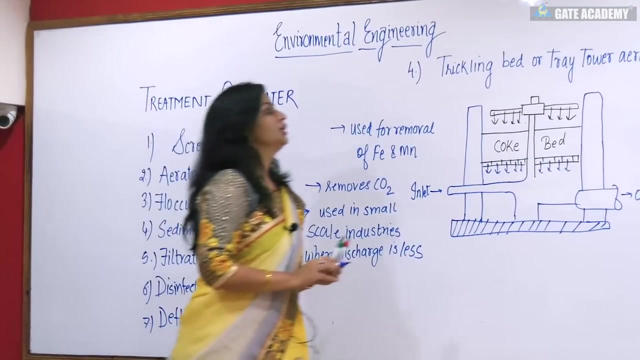 This is used in small scale industries- Okay, Okay, Okay. This is used in retail. Okay, Where the discharge is very less. Where discharge is less. Now, what is the mechanism? You can see this trickling bed or tray tower filter. what happens is water is made to pass. 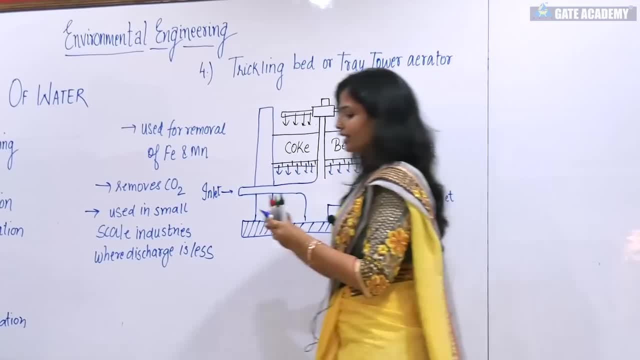 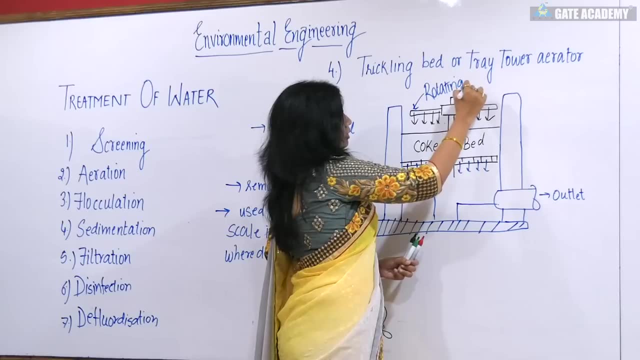 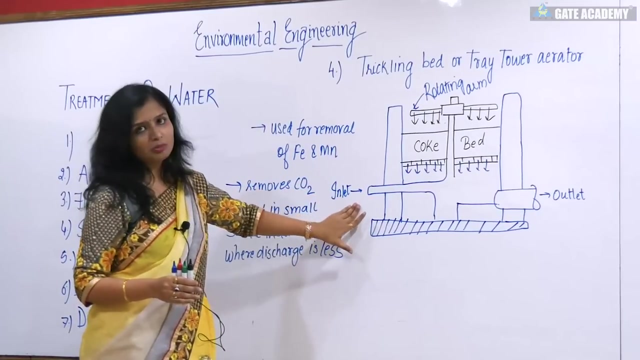 through the inlet, then it is made to pass, then it comes to the rotating arm. This is the rotating arm. Okay, Okay, Here water is made the treated water. after the screening has been done, it is made to pass through the inlet and after the passing through the inlet, it goes to the rotating 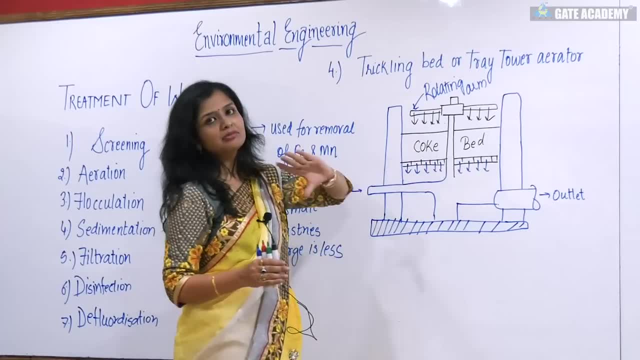 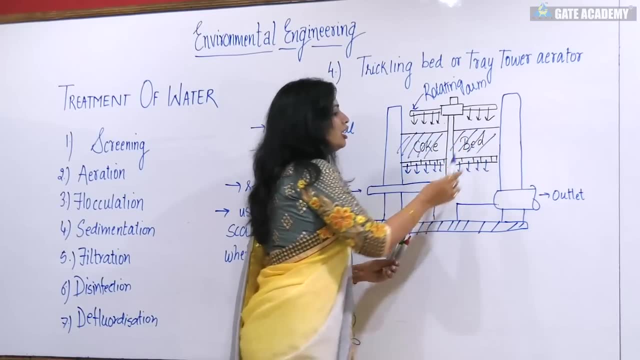 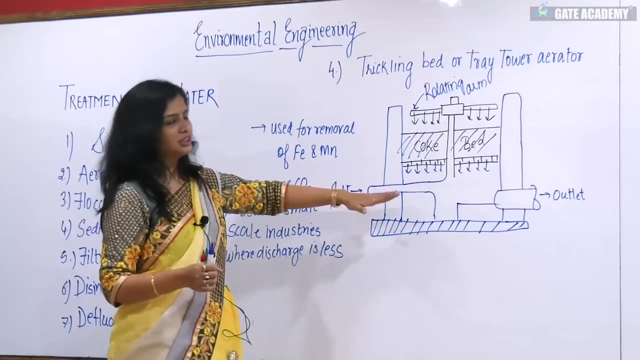 arms and after that it is sprinkled. the water is sprinkled and is made to come in contact with oxygen. You can see the coke bed is here and perforated pipes, we can say, are provided so that water could come in contact with the oxygen. 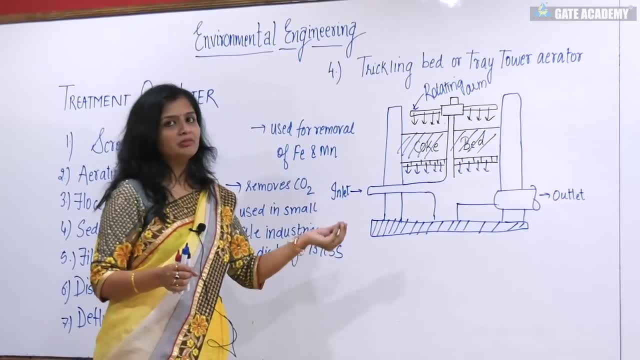 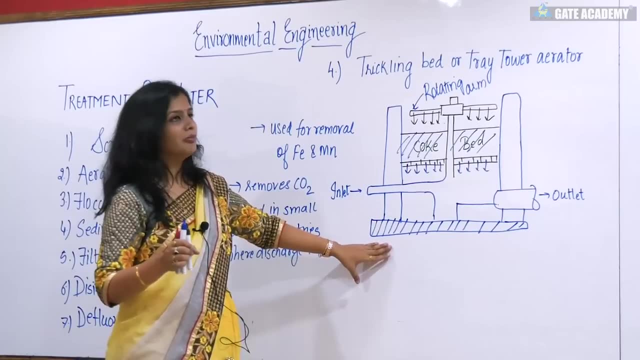 Basically, every mechanism of aerator is either through mechanical means, by with the help of motors, or with the help of freely following of water. anyways, we have to just make the water to come in contact with oxygen. So here also, with the help of coke bed we have, and with the help of the rotating arms, 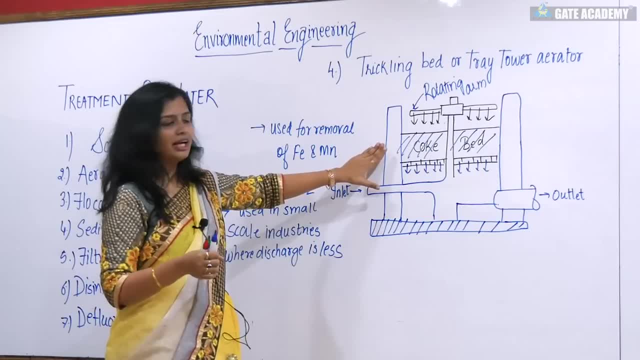 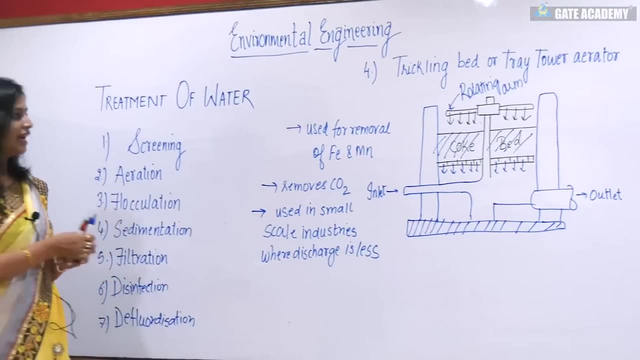 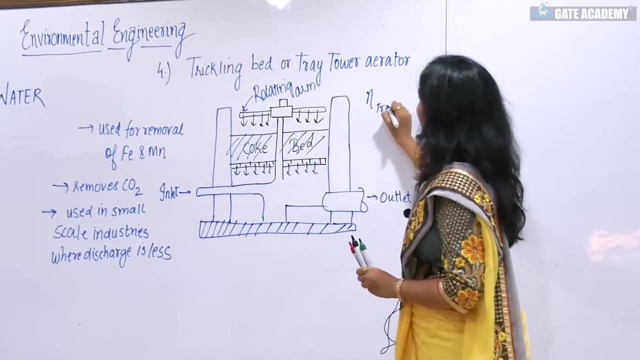 and the nozzles, We have made the coke bed, We are making the water to come in contact with the oxygen and then the treated water is made to pass through the outlet, Basically, as far as the efficiency is concerned, so the efficiency of this trickling tray tower, 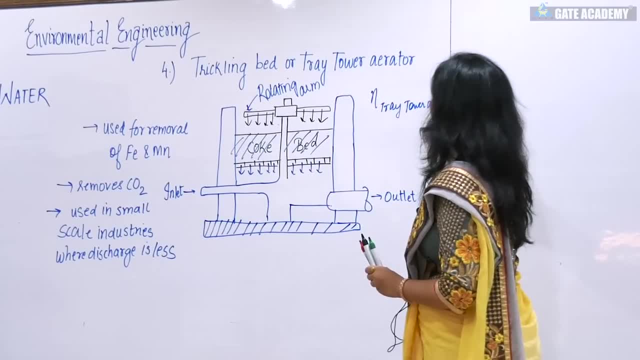 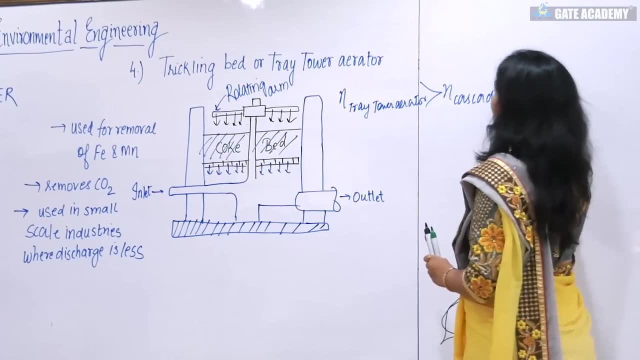 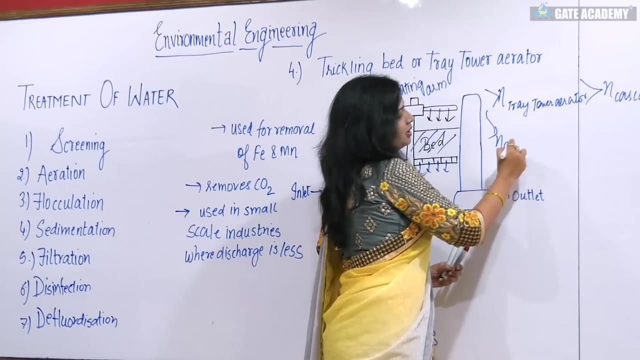 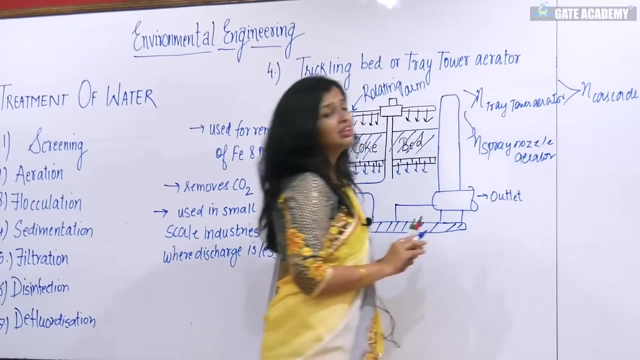 aerator is greater than the efficiency of the cascade aerator. however, its efficiency is less as compared to the spray nozzle aerator. So the ideal aerator which should be used is spray nozzle, but as far as economic point of view is concerned, instead of using this, we use cascade aerator. 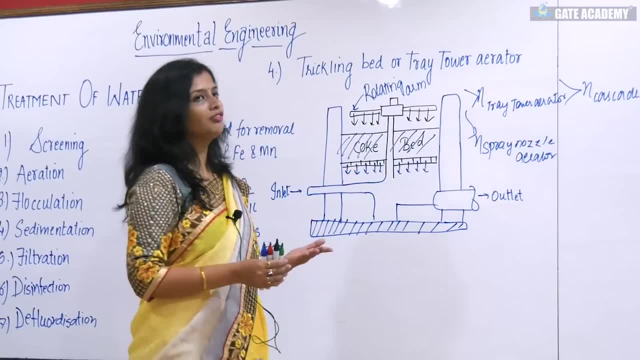 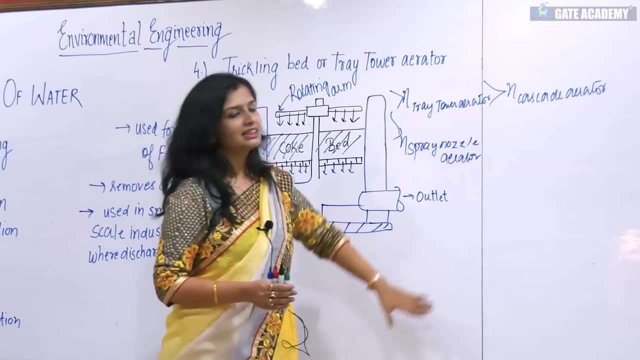 But if there is a small scale industries or where the quantity of the amount of water to be treated or the discharge is less, we can use tray tower aerator, as its efficiency is greater than the cascade aerator. Now we completed the screening part. 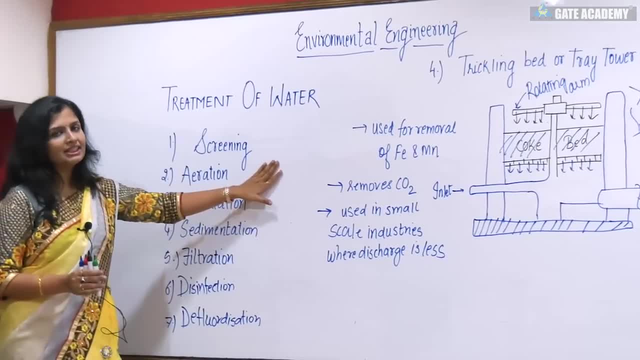 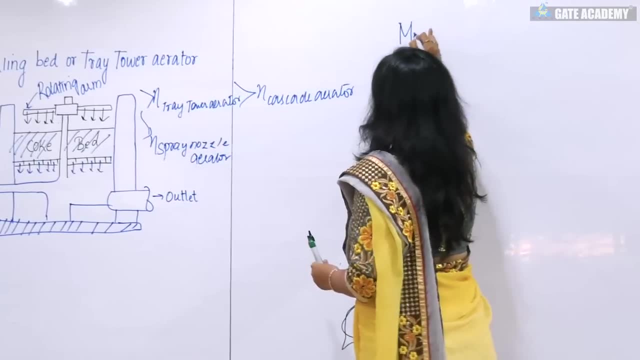 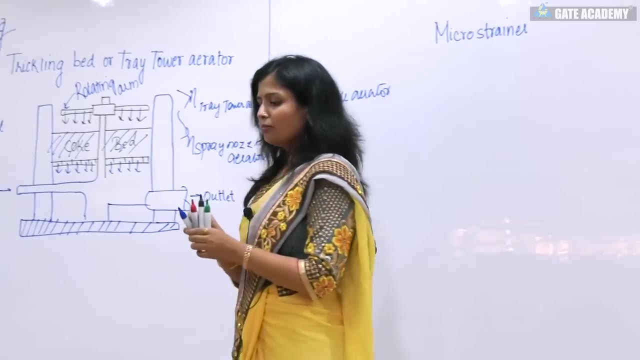 We completed the aeration stage. We completed the aeration stage. We completed the aeration part. But one thing: in screening there is a term: micro strainer. micro strainer. now, what is this micro strainer? What happens Sometimes if you are collecting a water or you have stored the water somewhere, then 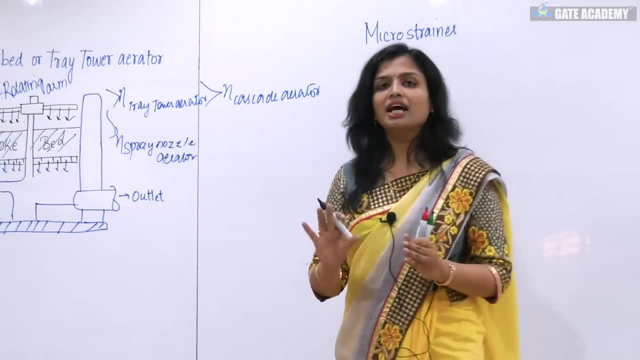 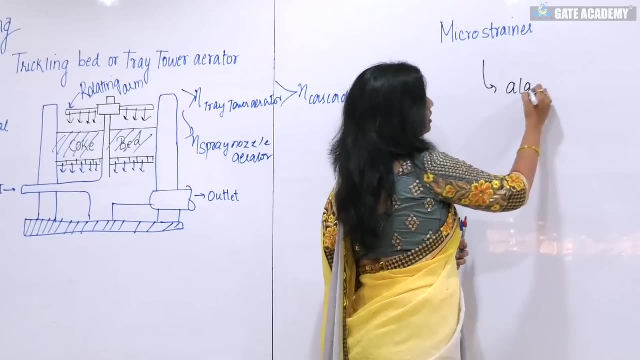 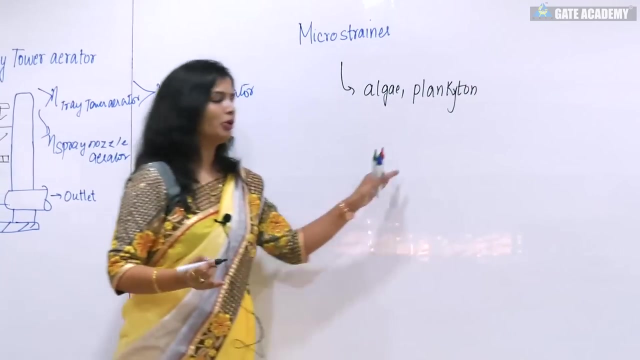 you can see there is no large suspended particles or large floating matter. there is no sort of these matters. But you can see common particles, Common particles, Common particles, Components, like all guys: plankton, Plankton in water, phytoplankton. 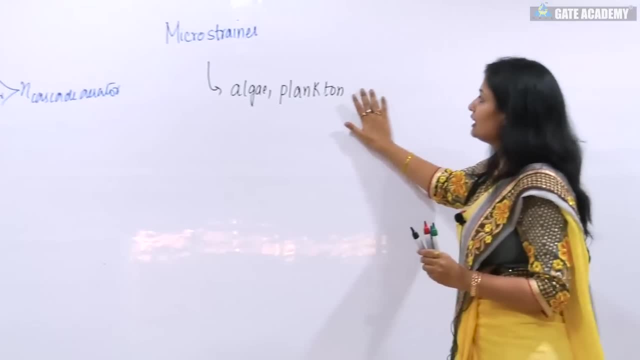 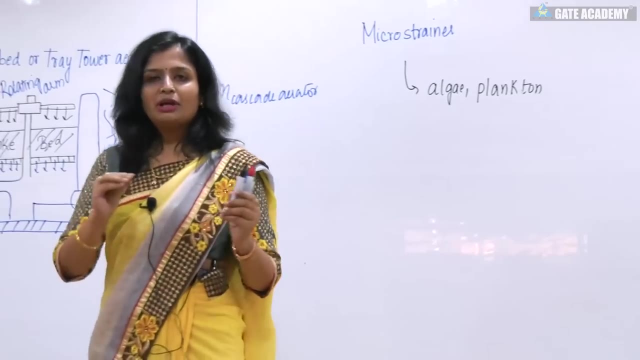 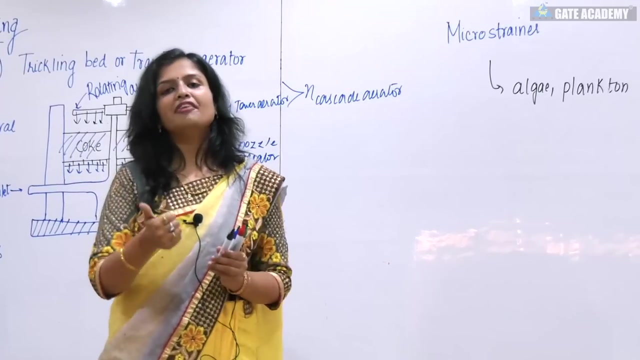 So plankton in water. so when you see this- and plankton in water, what you see- You want that it should not be present, Because if you take this water, the all guy components in water in filtration chambers, then it is not sufficient. 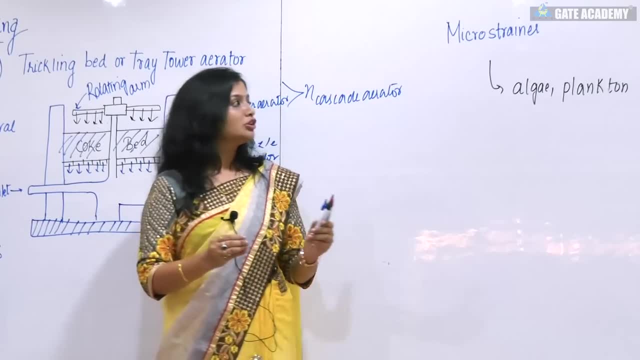 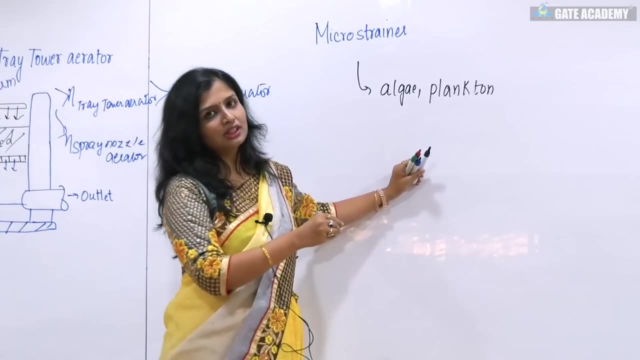 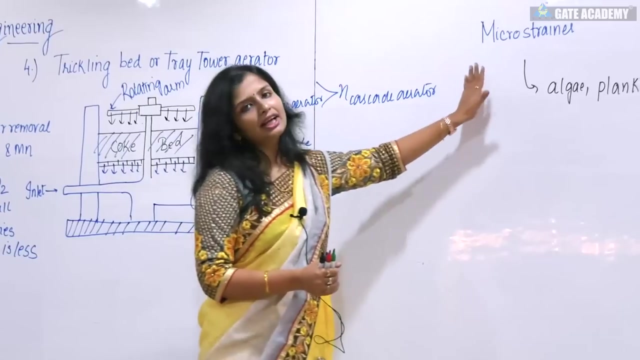 So because of this we use microstrainer. best place, ideal place where you can keep microstrainer. when you will study filtration, then you will study rapid sand filter and slow sand filter filtration unit Before that. if you put microstrainer there, then what will happen? whatever alga or plankton, 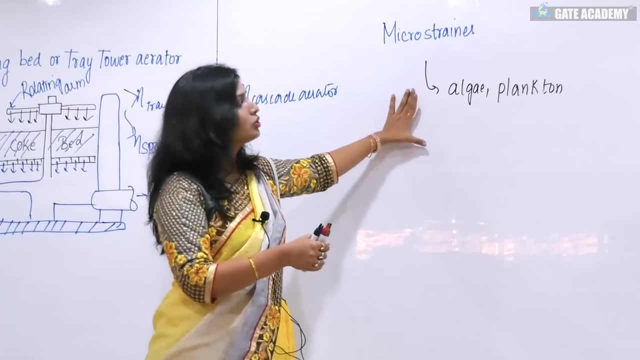 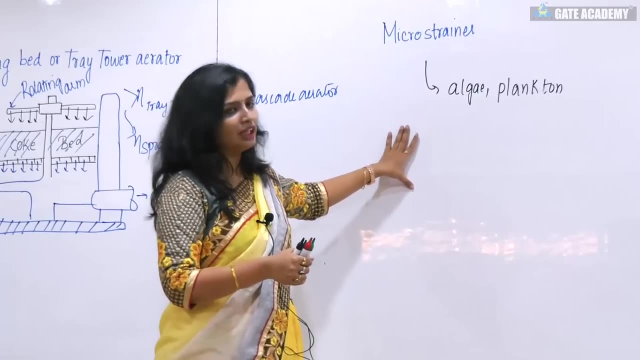 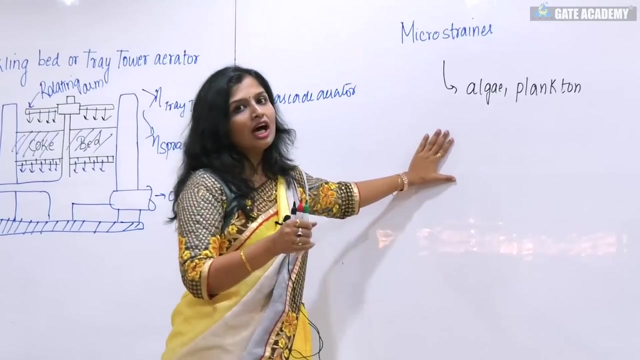 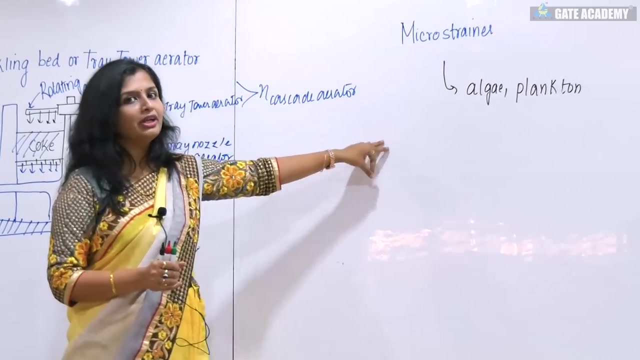 are present in stored water, it will capture it and after that the remaining water will be sent to filtration. If you put it before slow sand filter or rapid sand filter, then your efficiency increases as much as 50%. So basically, this is also one of the part of the treatment unit. in places where the 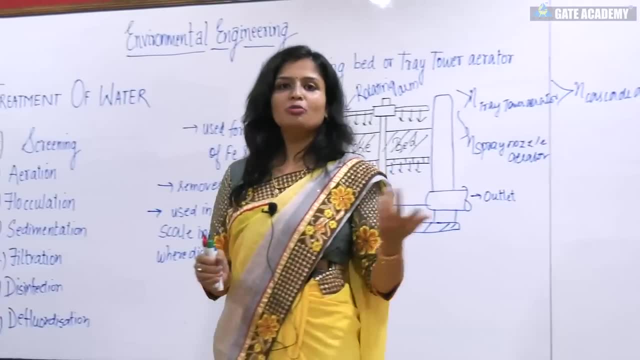 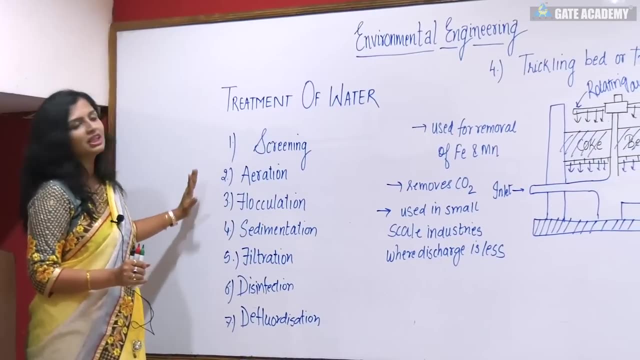 growth of algae is more. then we have to use microstrainers for water treatment. So we have completed this screening part. I hope you are clear with this: coarse screens, fine screens. So we have completed the aeration part. now comes the flocculation part, but before 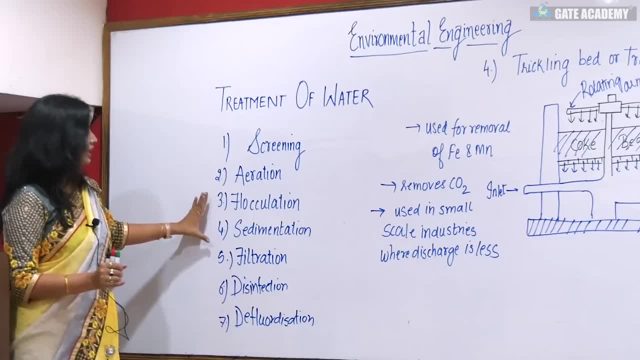 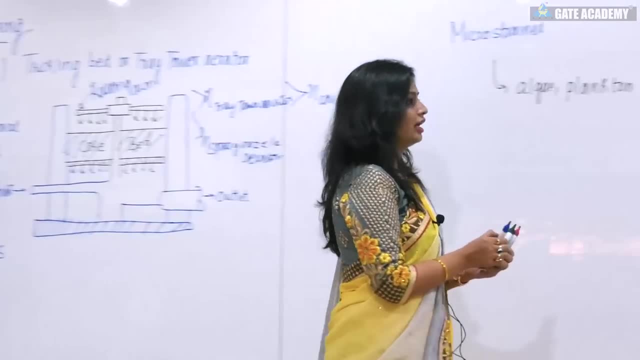 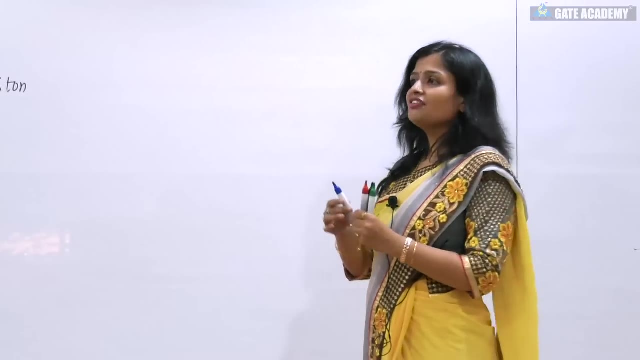 discussing the flocculation, I will make you to understand the coagulation flocculation together, but let us starts with the sedimentation part, because after understanding the sedimentation part I hope you will understand the flocculation and coagulation, if sedimentation can be done. 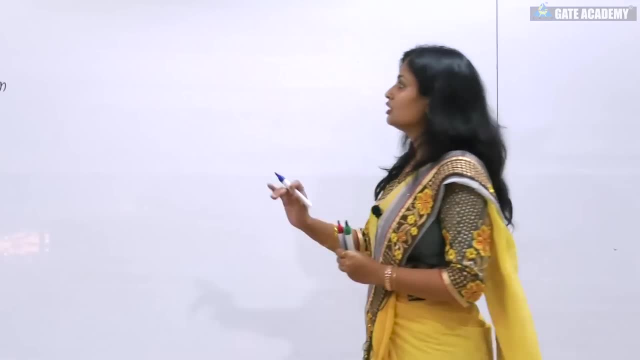 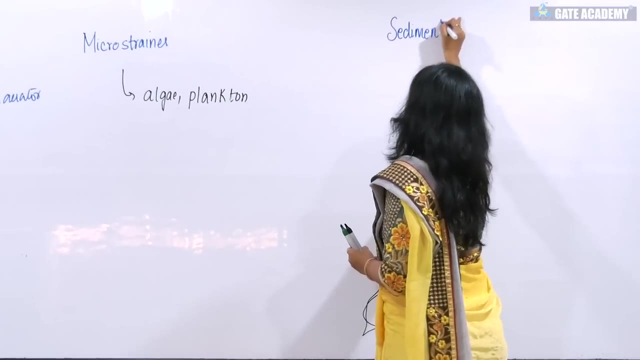 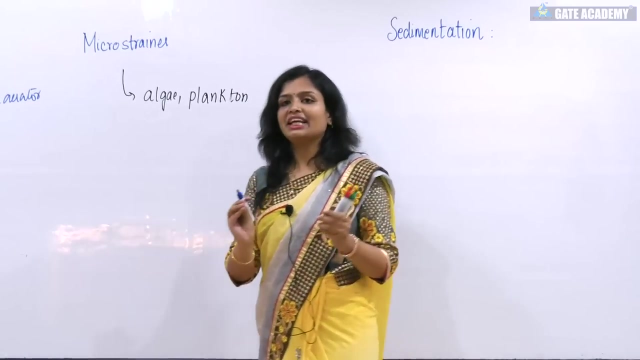 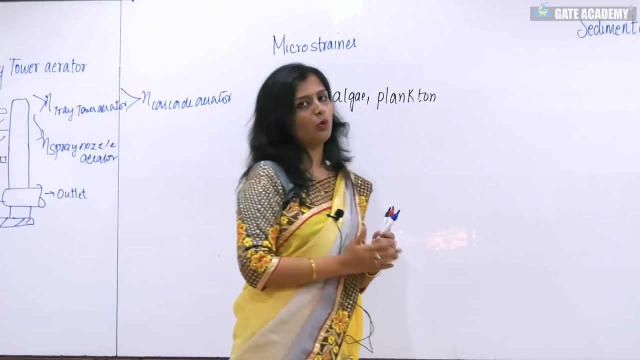 why there is a need that we should flocculate the particles. So, basically, now we will be dealing with the sedimentation part. We will be dealing with the sedimentation. What does sedimentation means? It means that the large suspended particles are made to settle in water. 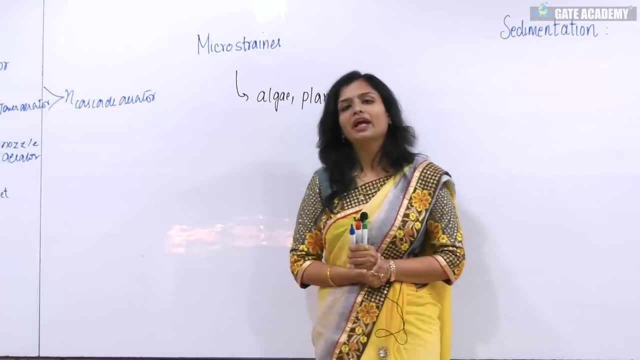 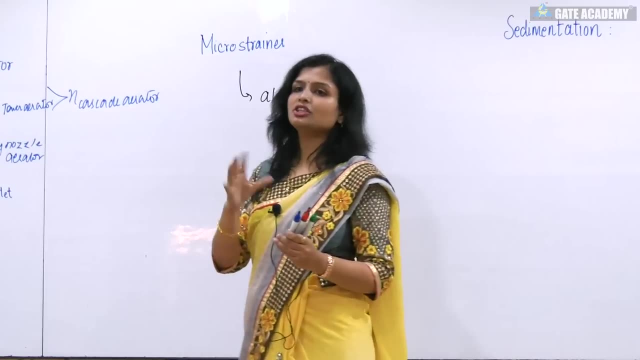 When we have done screening, we have said that large floating matter has to be removed, that we keep it inclined so that its flow area increases, velocity decreases and the floating particles gets settled. Now, when we have done the screening of water by applying oxygen to it, we have controlled 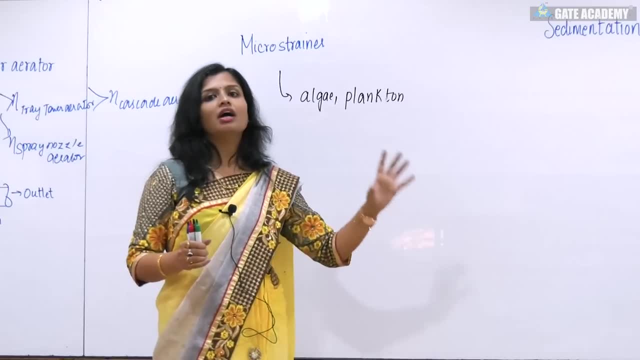 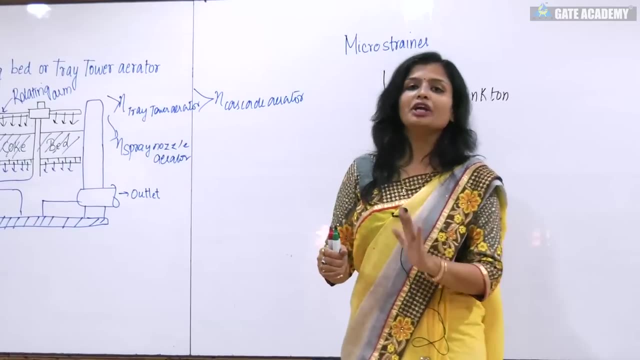 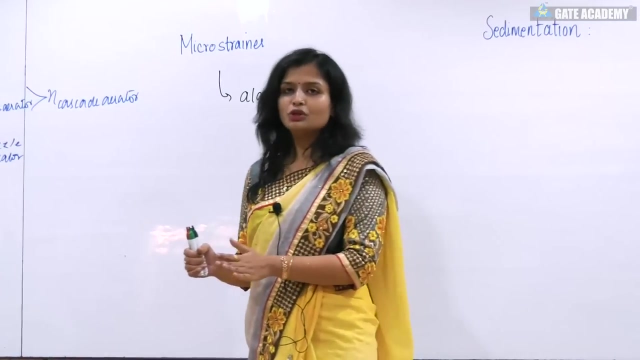 the harmful colors, odours, precipitated harmful compounds. After that we have done the next treatment in sedimentation. In sedimentation, those very particles settle in the water whose specific gravity is more than water or whose density is more than water. 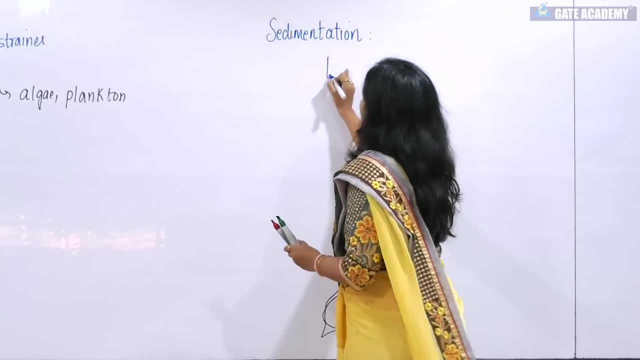 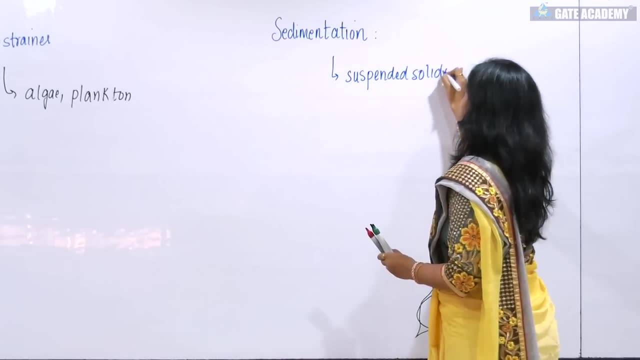 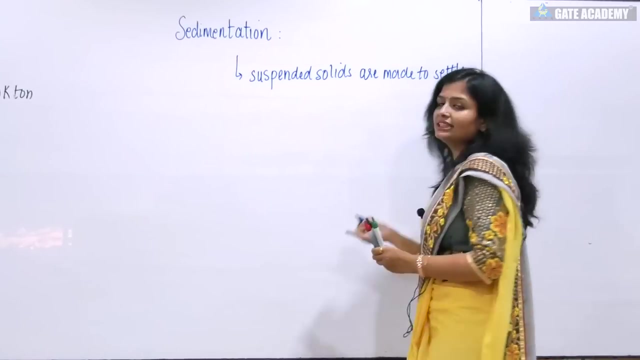 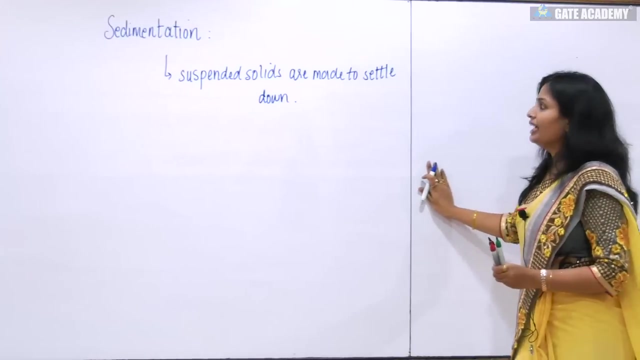 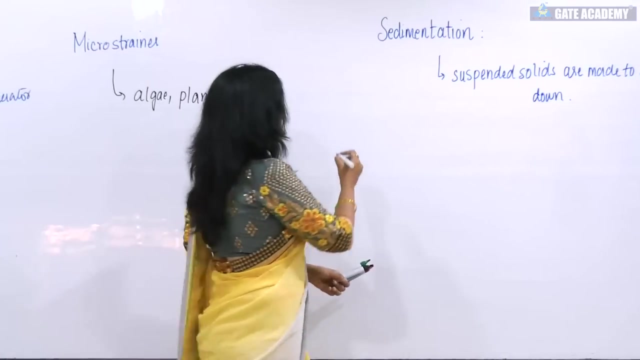 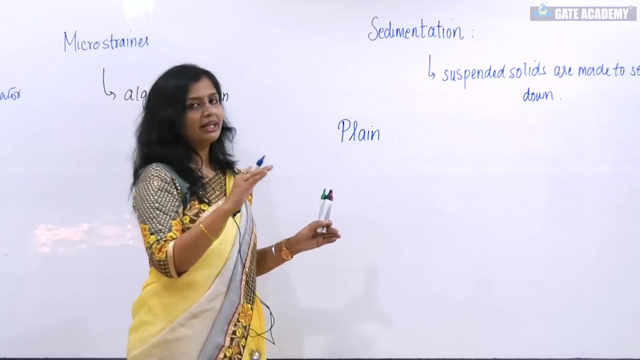 And in this what we do is suspended particles or suspended solids, are made to settle down. And who will settle down, the density of which will be more than that of water. Now for sedimentation. you have two types of sedimentation. One is plain sedimentation that you have only, given sedimentation, collected the water and the density of which will be more than that of water. it will settle down. 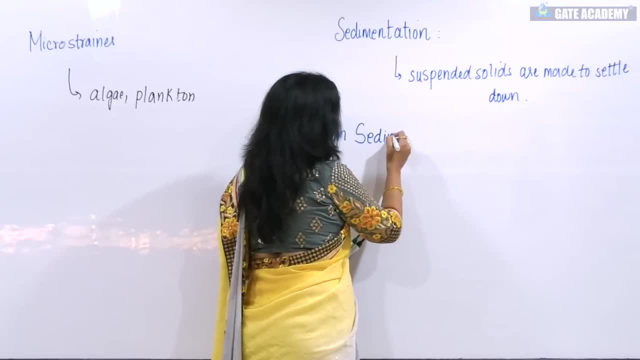 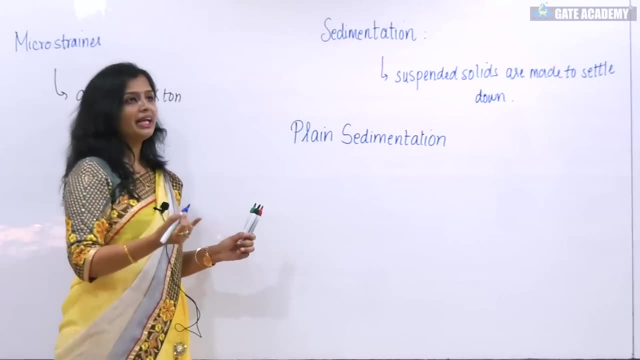 And one is: sometimes there are so many components in the water that they do not fall down quickly. they keep floating. there are minor particles which keep floating. You may be able to see it with naked eye, but if you want it to settle down in water at one place, then it does not settle. 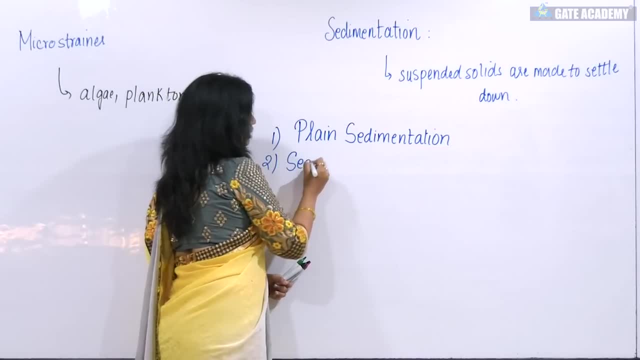 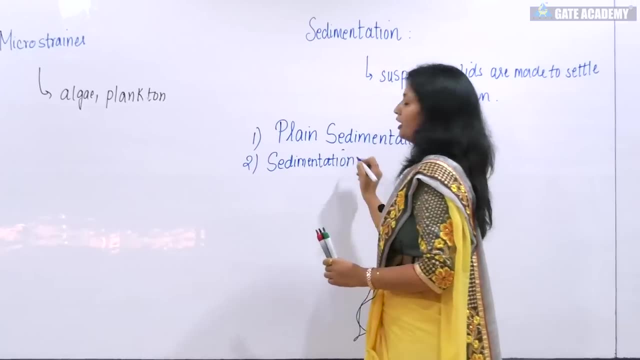 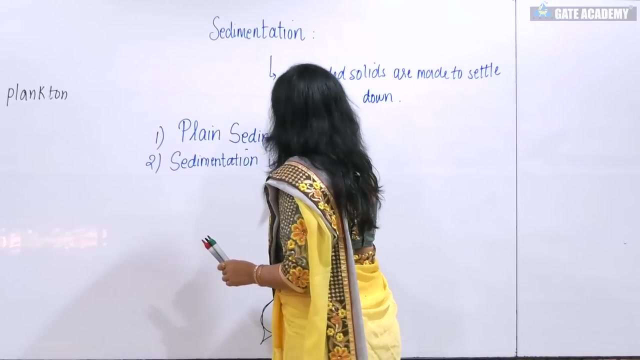 So in that case what we do is sedimentation with coagulation. This is very important part of sedimentation because it has numericals, so your concept should be clear. Then only you can solve the numericals. Sedimentation with coagulation. 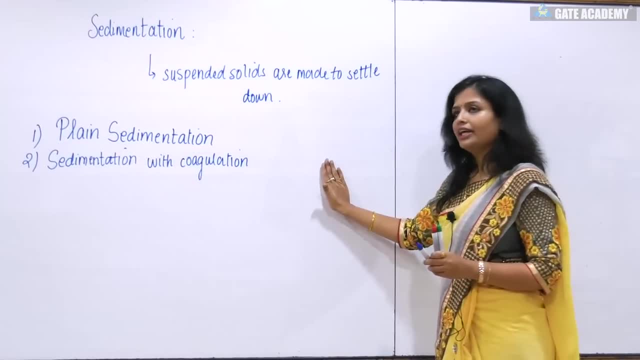 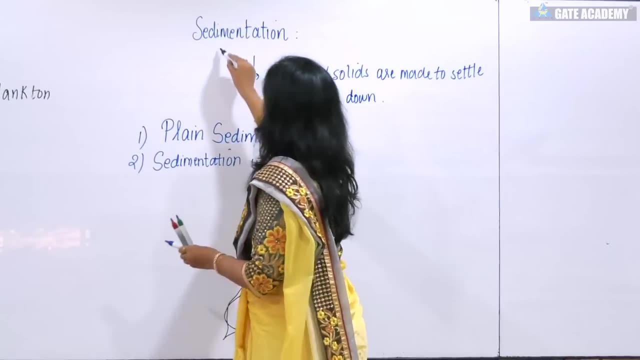 There is design part of plain sedimentation. How much to overcome in that Overflow velocity, settling velocity? we will deal with all of them now. So sedimentation is basically divided into two parts: Plain sedimentation, sedimentation with coagulation. 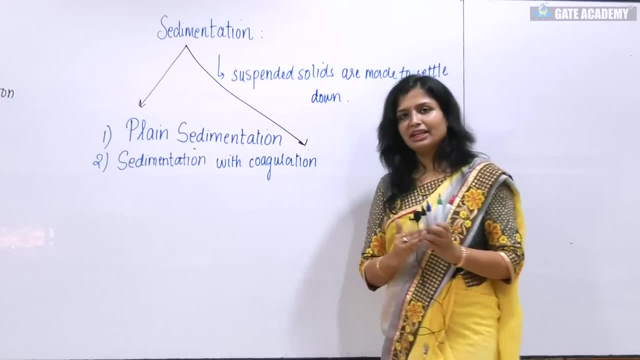 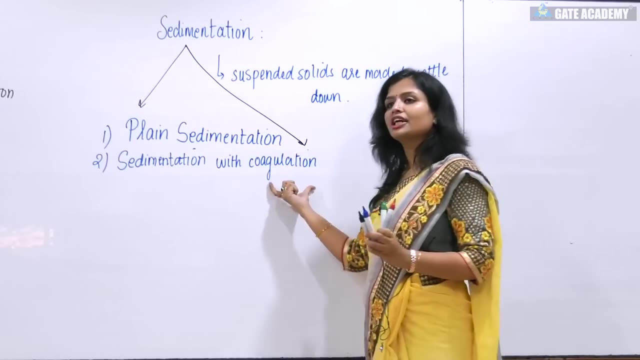 First we will be focusing on plain sedimentation. Once we will complete the part of plain sedimentation, after that we will come to sedimentation with coagulation: Where. what is coagulation, what are coagulants and in which coagulants are used, their formula. 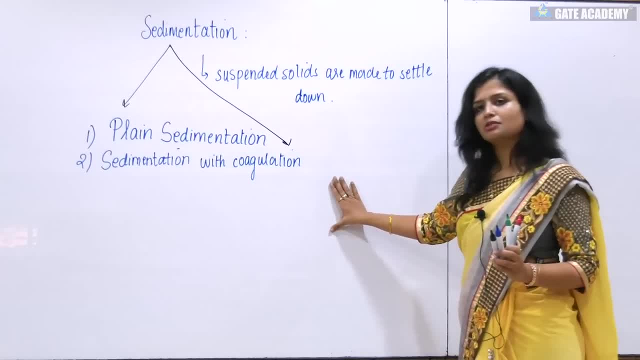 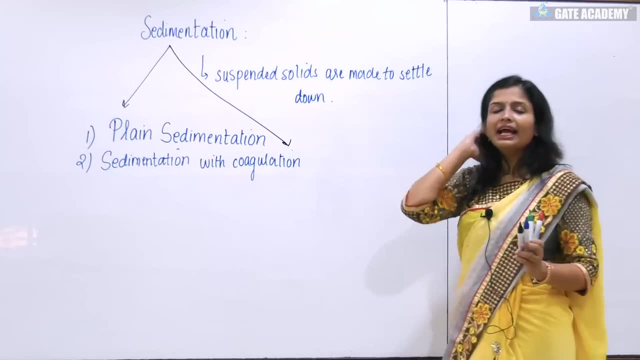 we will discuss all of them, Even how many doses should be provided, how to calculate it- that too we will study. in sedimentation with coagulation: How will we know how many coagulants we have to put in 1 liter of water? 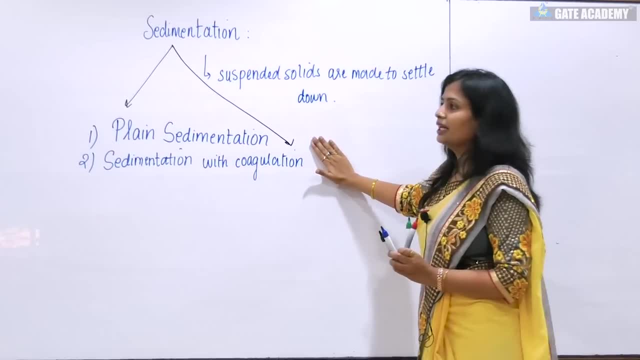 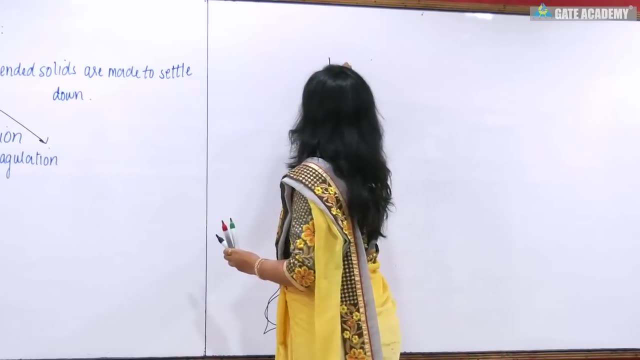 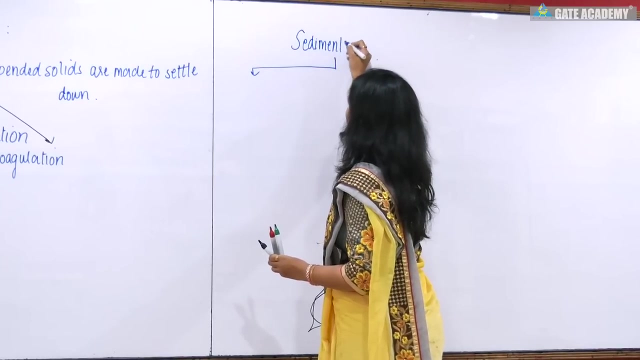 We will study all of this, But before that we will study plain sedimentation. we will study the designing of plain sedimentation. Before plain sedimentation tank, you should know one thing First: sedimentation tank is of two types. sedimentation tank is of two types. sedimentation tank is of two types. One is quiescent type, This is also called intermittent type, Intermittent type- And one is continuous type. So quiescent type of sedimentation tank means that in quiescent type you collect the water. 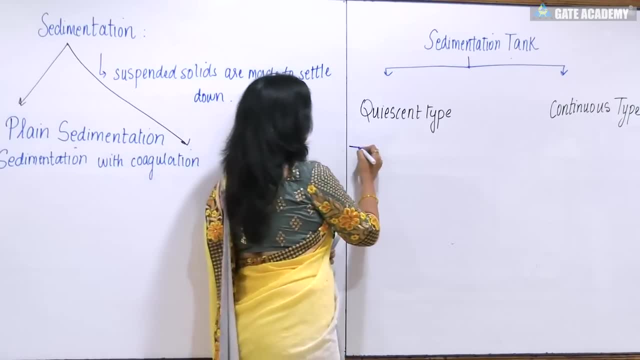 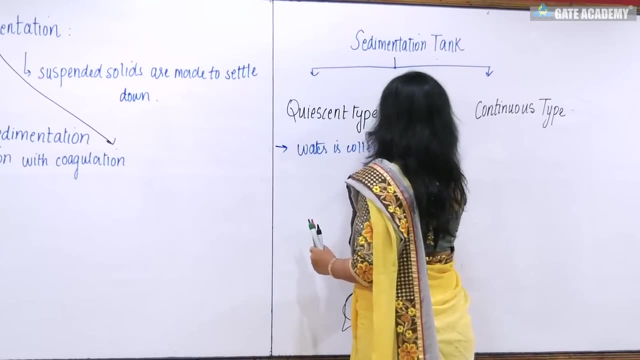 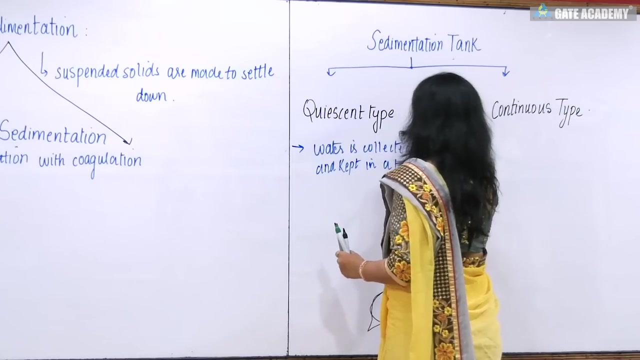 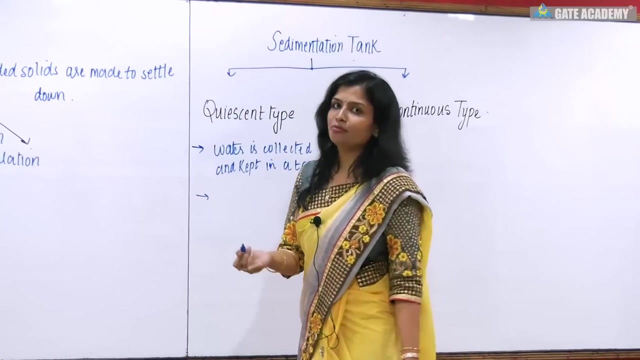 at one place and keep it Here. water is collected and kept in a tank. you can see You have kept the water in a tank. For how long? For as long as you have kept it. it is called detention time In environmental engineering. we do not say time only. 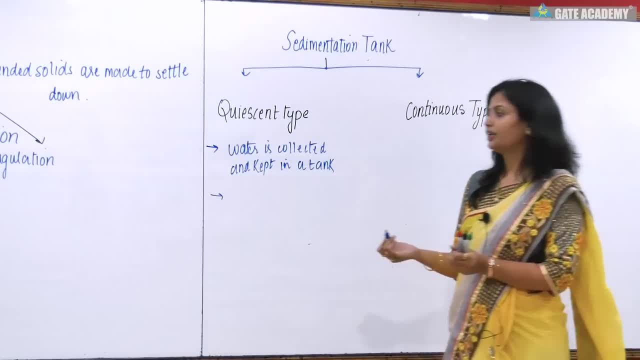 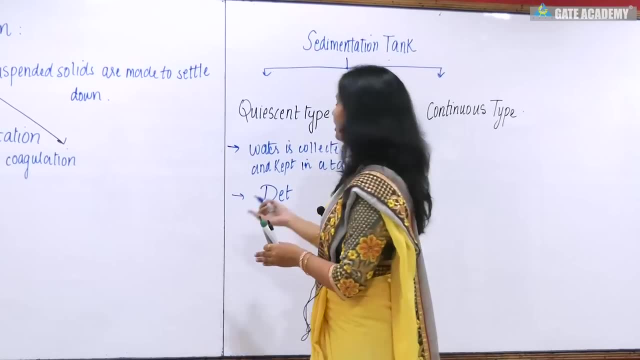 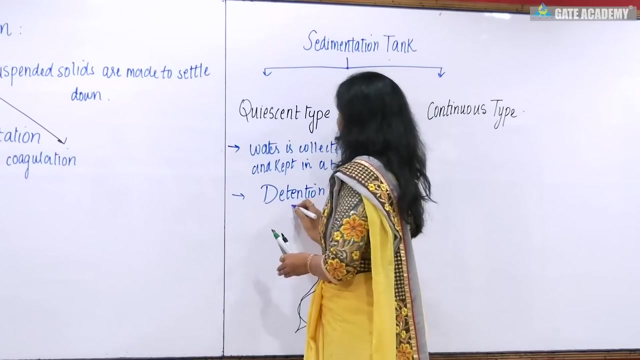 Whenever we talk about treatment units, we will say detention time. Okay, from today onwards, whenever you say to accumulate water or to treat in sewage, or to tank in plain sedimentation, we will say detention time. We will call it 24 hours, 24 hours. 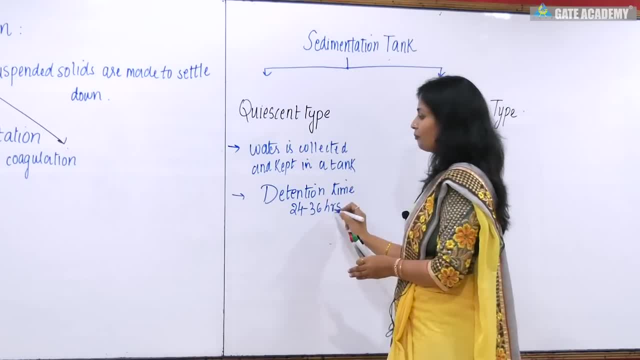 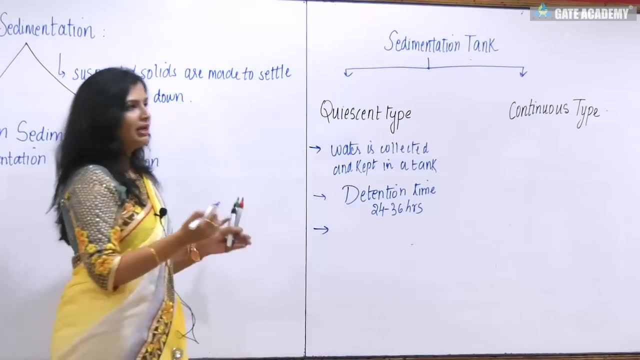 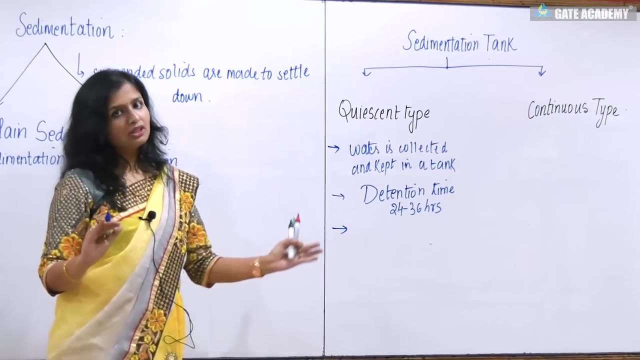 24 hours to 36 hours. water is kept in it. that water is not moving. the water is resting. the period of cleaning that is left. you have kept the water once, all the particles whose density was more than water. it has settled now to remove those particles. the time that takes. time for cleaning, the time which is required for period of cleaning- this is 8 to 12 hours- and how many tanks are required. for sedimentation tank, so minimum 3 tanks are required in quiescent type sedimentation tank, so minimum 3 tanks are required. 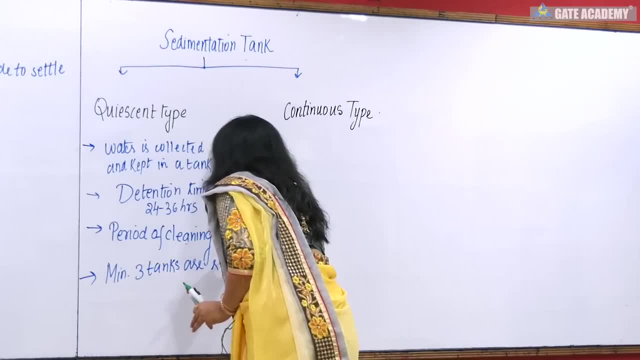 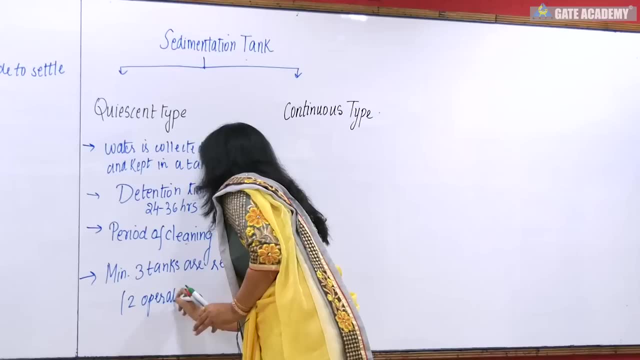 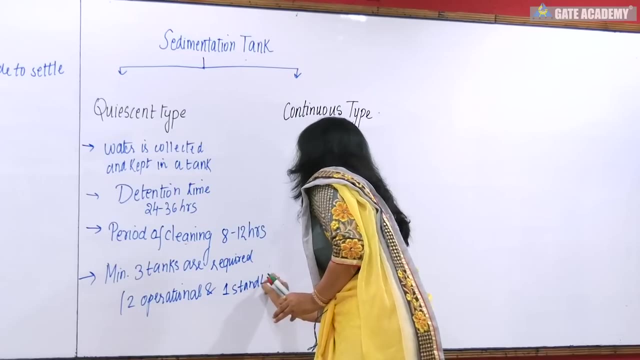 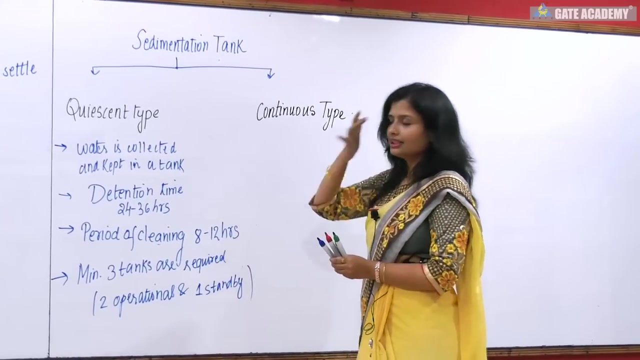 Okay, At least, out of which 2 are operational and one is in standby, and one is in standby. So these are the features of quiescent type. we collect the water and store it there. the detention time: we keep the water for 24 to 36 hours. 8 to 12 hours. So these are the features of quiescent type sedimentation tank. so minimum 3 tanks are required to remove the sludge. so we keep the water for 24 to 36 hours, so minimum 2. tanks are required to remove the sludge. so we keep the water for 24 to 36 hours And for this minimum 3 tanks are required, out of which 2 should be operational and 1 should be for standby. nowadays we do not use quiescent type, because you are seeing, 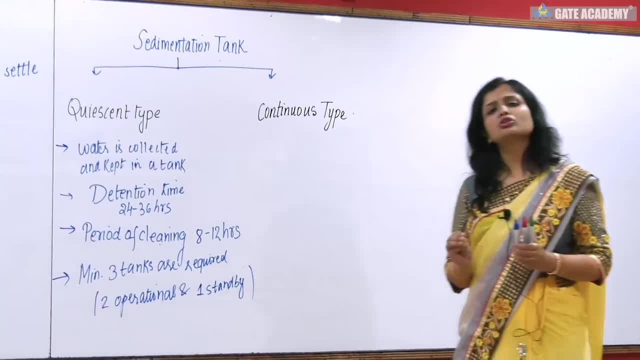 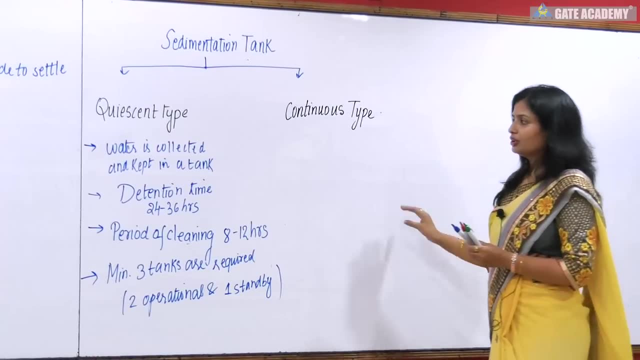 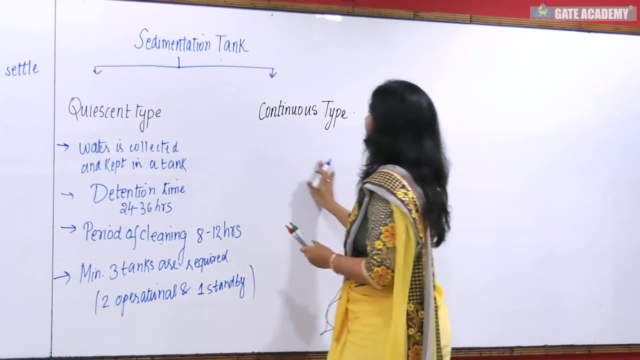 that so much period of cleaning is required. manpower is also being applied. okay, so nowadays we do not use quiescent type sedimentation tank. it has become almost obsolete. now, when we talk about continuous flow type tank is that you are making the water flow, but at a reduced velocity. its sub-categorization. 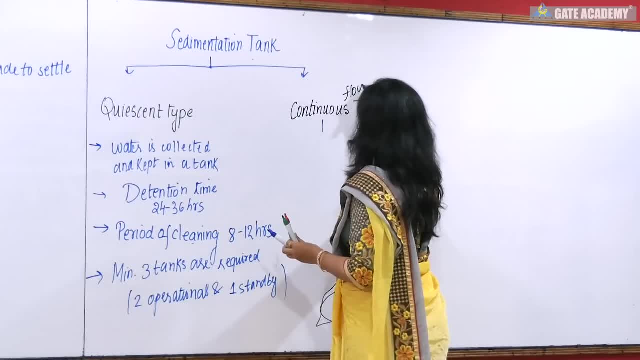 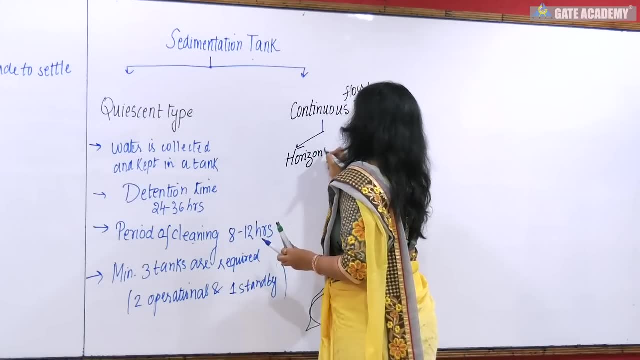 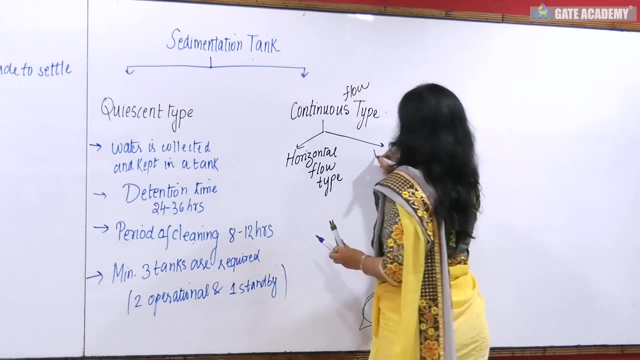 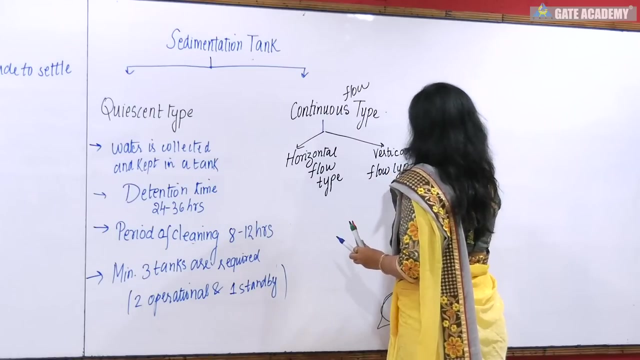 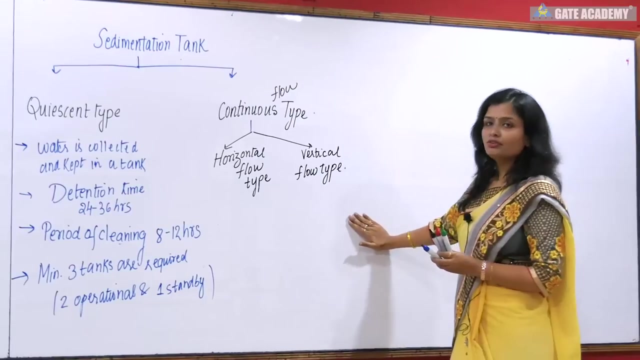 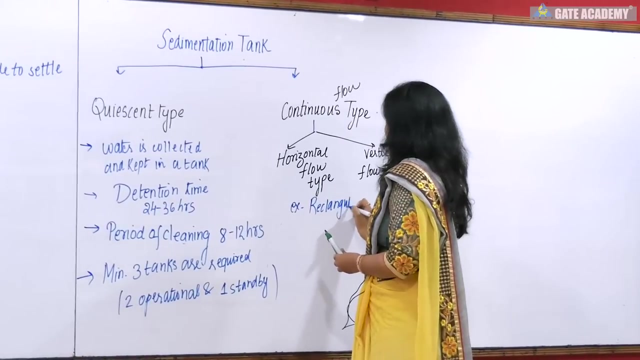 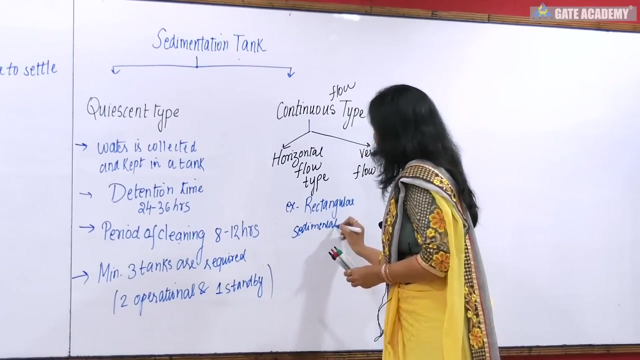 is continuous flow type. its sub-categorization is horizontal flow type and vertical flow type. The example of horizontal flow type is rectangular sedimentation tank, which is used very highly, and we prefer to use rectangular sedimentation tank And the example of vertical.